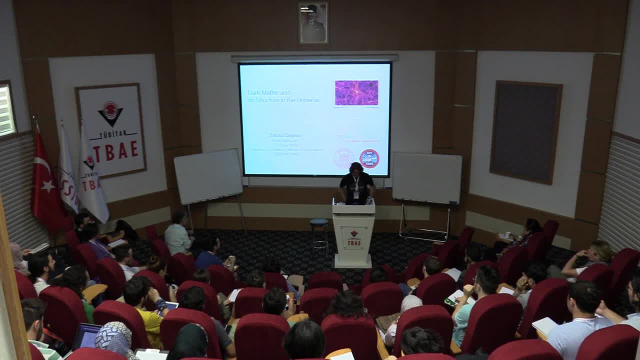 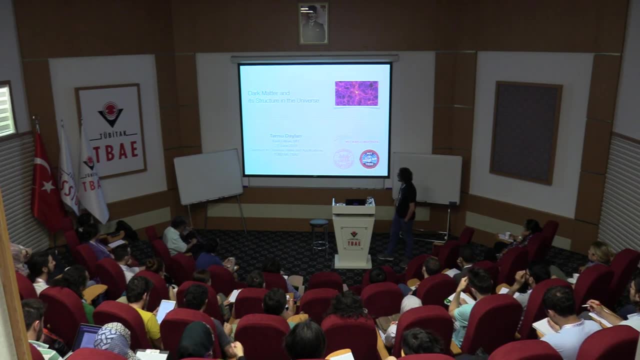 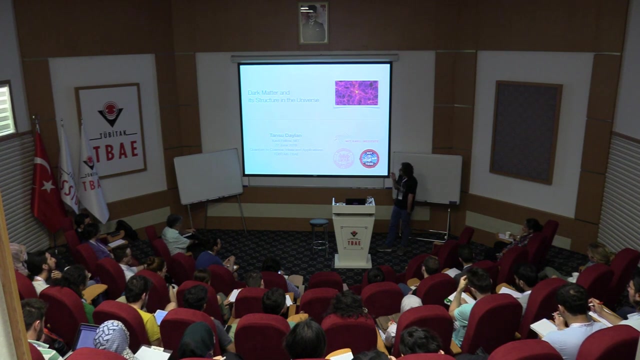 but I hope I won't touch them. They're too close to the laptop. Okay, so today we will switch gears. Yesterday I gave a talk about exoplanets. today and tomorrow It will be a very different topic, In fact, I mean, tomorrow will be even different from today. So today the idea is to introduce the idea of dark matter. 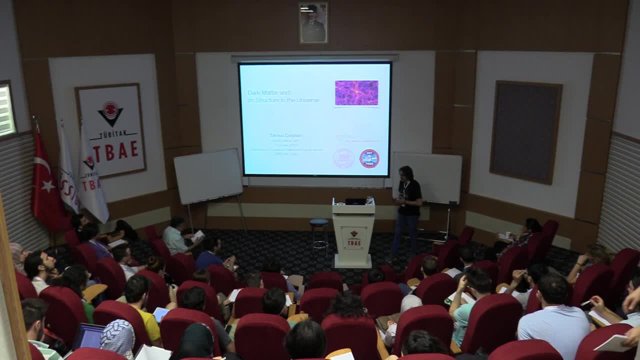 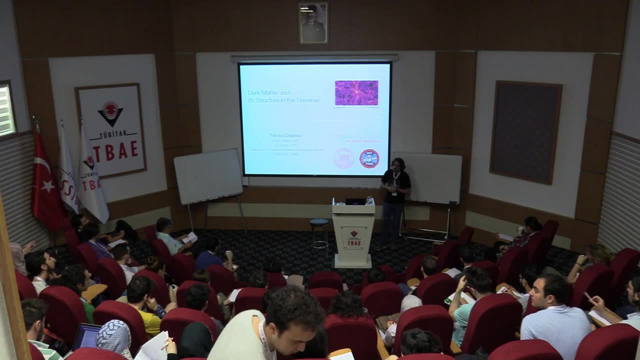 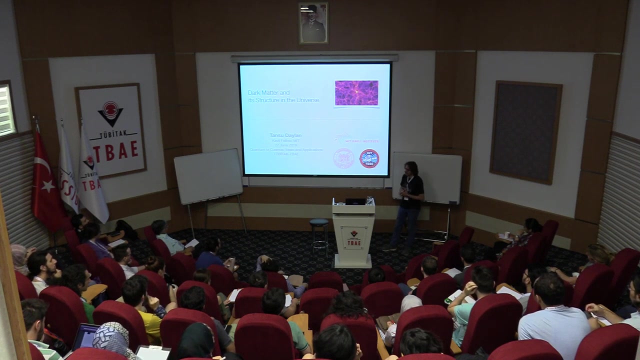 pretty much lay out the problem and then discuss some solutions to it in the cosmological context. I won't go very much into the particle physics details of the problem because we have a special lecturer, Tracy, who is my academic sister. We share the same advisor. She'll be in town in a few days and she'll give a couple of talks. 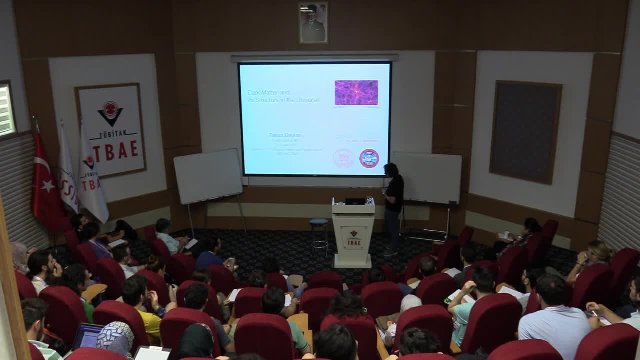 one of which we'll cover The particle physics aspect of the dark matter problem. So I'm not going to touch that part very much, except the fact that I will discuss the GeV excess problem. So here's just a quick outline of the four lectures. 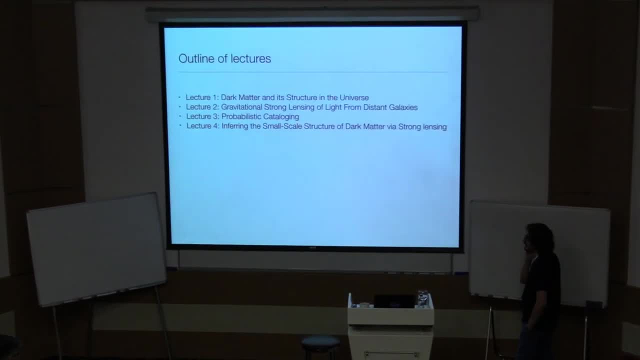 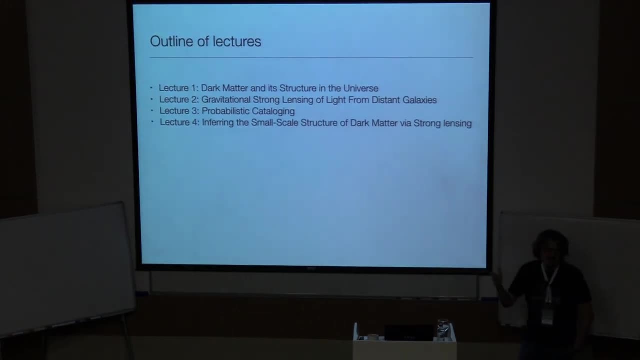 that I will be giving, So today's lecture, the lecture one, is about dark matter and its structure in the universe. So by structure I mean spatial distribution as a function of time. We will discuss various aspects of the structure formation and how dark matter is involved in this And second lecture, which will be the second lecture of today. 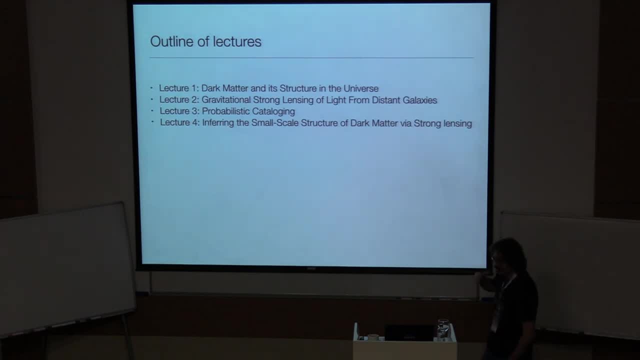 it will be about gravitational strong lensing, Or in fact, I will start with gravitational lensing as a general idea and then go into strong lensing, the lensing in the strong regime, And then, tied to astrophysics, just show some pictures about how strong lenses 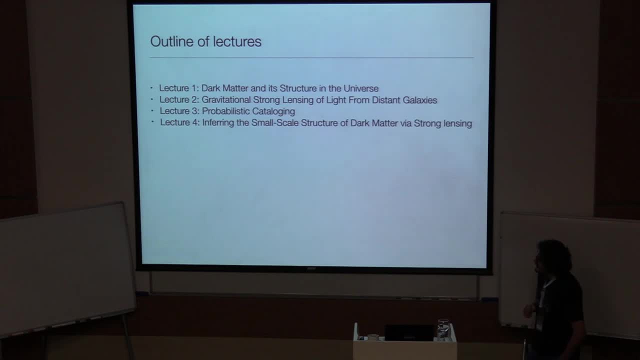 actually come into existence in our universe. Lecture three, which will happen tomorrow afternoon, it will be about probabilistic cataloging. I'm sure it doesn't mean anything to you when I say that, And it's all fine, because it's a recent idea that we are trying to introduce into the astrophysics literature. 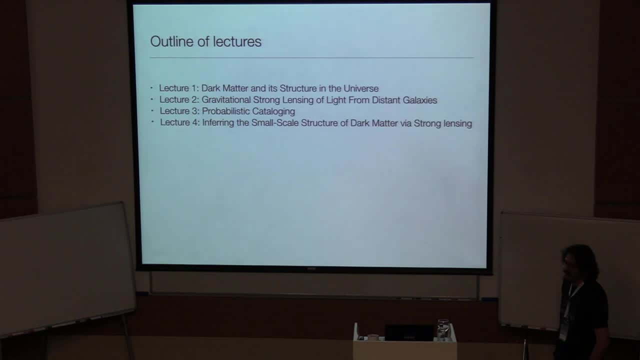 rather astro-statistics literature. So lecture three will be mostly about statistics, So it will contain minimal physics and maximal computer science And statistics. So it will be a different flavor and kind of lead the way into lecture four, where we will bring ideas from lecture one, two and 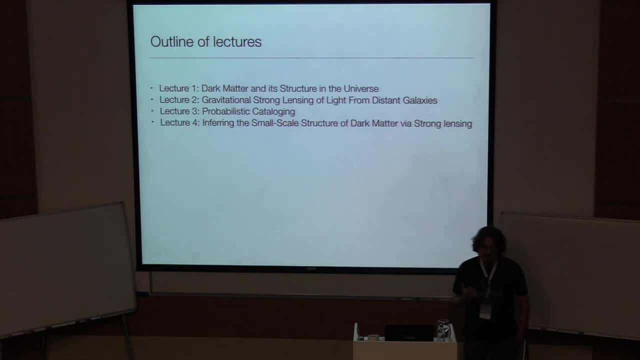 three together to try to answer some questions about the small scale structure of the dark matter. So it will contain pretty much materials from all the three previous lectures And hopefully by then you will understand what probabilistic cataloging is and why it's important. 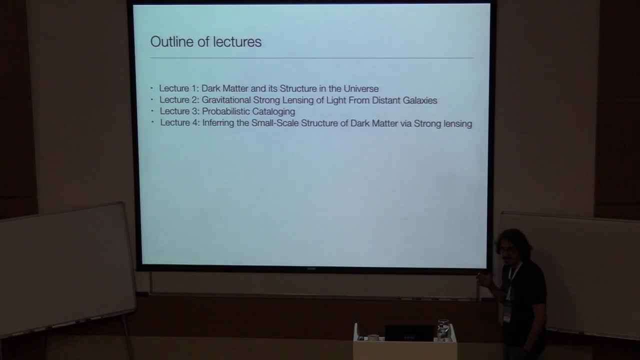 So these four are the lectures Now. yesterday I was expecting actually more questions during the lecture. So please, please, do feel free to stop me and ask questions. This has to be interactive, otherwise I just can't see or probe how much information is being. 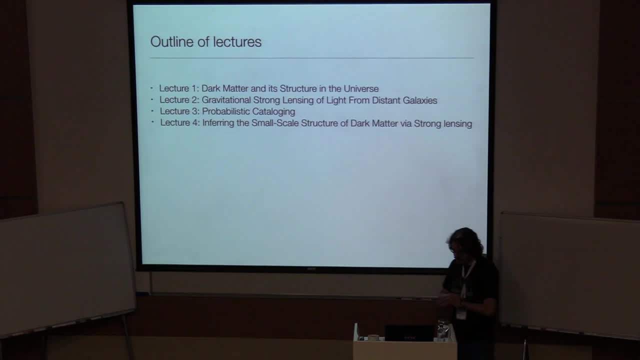 transferred. So, yeah, let's make this as interactive as possible And I will certainly leave some time at the very guy end for questions I have. I did not plan for 50 minutes lectures, I planned for slightly less, So there will be ample time for discussions by the end. 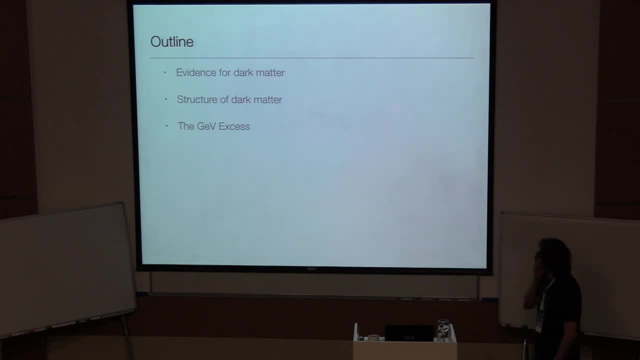 So now coming to today's lecture, the lecture one about dark matter and its structure. So there will be three components to the lecture. First, I will talk about evidence for dark matter, basically why we think there is something called dark matter. Second part, I will talk about its structure. 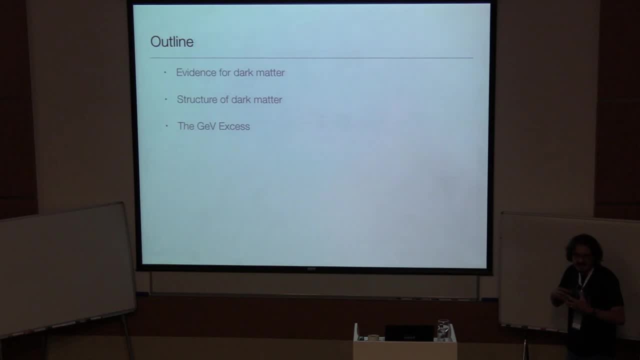 As I said, it's the spatial distribution And they are tightly connected And hopefully that will become clear why. And in the last part I will talk about the so-called GEV access. Some of you may have heard the idea. 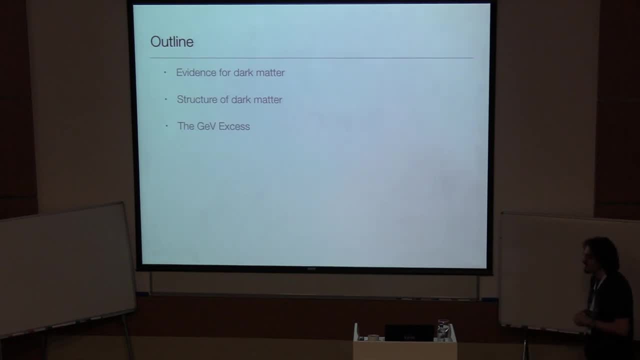 Probably many of you who don't think about dark matter on a daily basis haven't even heard the idea. That's totally fine as well. I will talk about what it is first and why it's important. It's one of the problems I've worked on during my PhD. 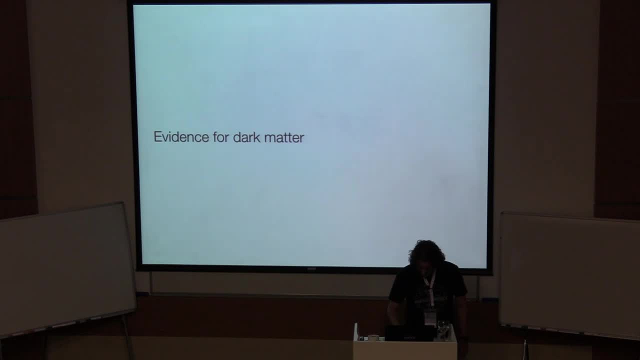 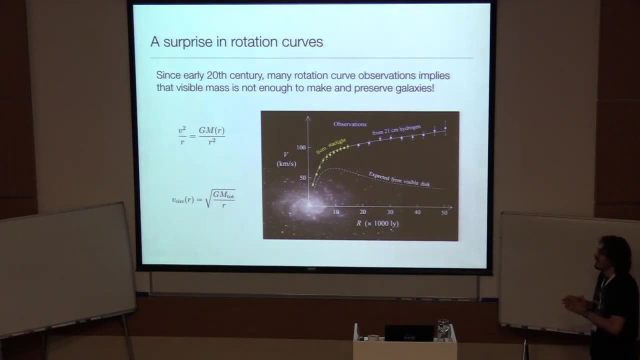 So coming now hierarchically going down to the evidence for dark matter, So I will start the lecture pretty much going a century earlier. So think about early 20th century, where people were just even realizing that our galaxy is not the only galaxy in the universe. Back then people were just calling what we call today as galaxies, just nova, or basically like when they saw new objects, or just like nebulae, whenever they didn't understand what that meant. But early 20th century evidence started to build that there's additional galaxies. 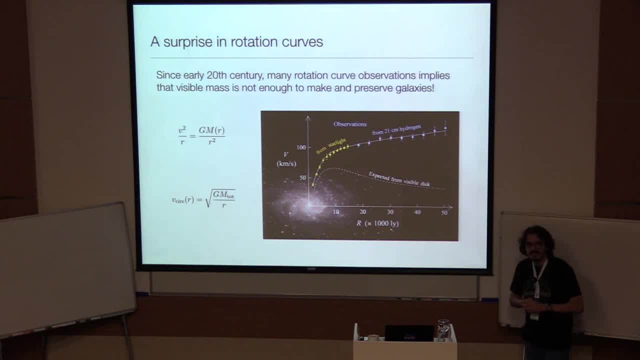 In fact, later, billions of them, And people started asking questions like: how do we do this, How do we do this, How do we do this? How do the stars in those galaxies move, Including our own, obviously? I mean the first order question you should ask. 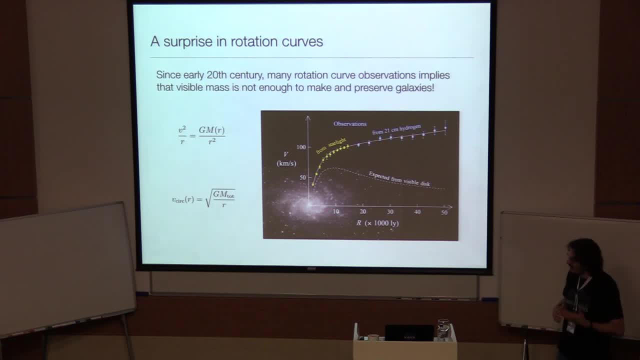 is: how do the stars in our own galaxy move? But then you can ask that question for other galaxies as well. So in this plot, for example, you see an example answer to such a question, where, on the x-axis, you see basically: 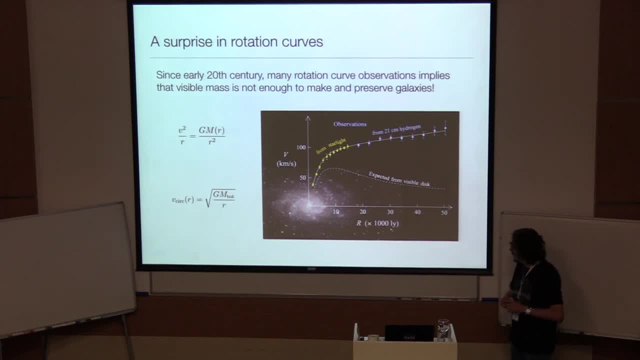 the radius from the center of the galaxy And on the y-axis you see the circular velocity in kilometers per second, in units of kilometers per second, And there's a bunch of data points and two theoretical curves on the plot. So if you just concentrate on the yellow data points, 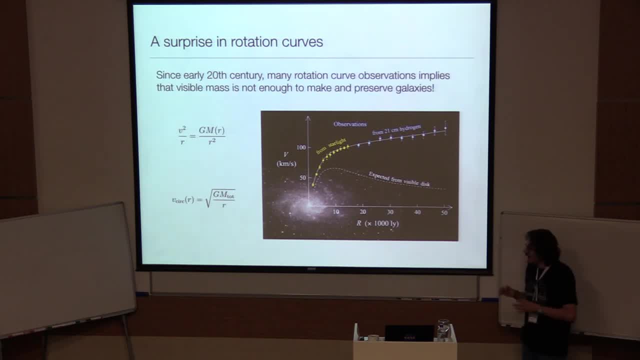 those essentially come from starlight. So you people, I won't go into details very much now, but things will progress. So they just measure somehow The velocities of the stars And they make up the yellow data points, with certain uncertainties involved. 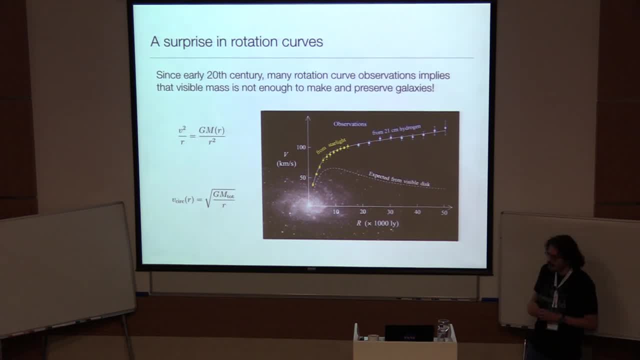 And shown with the pale blue is the same type of data, but those data points come from a different source. They come from 21 centimeter emission of hydrogen, But eventually you see that they are actually increasing. Now if you just stop and think about very basic Newtonian 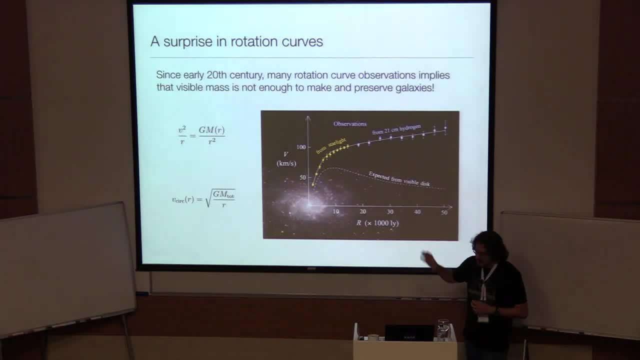 dynamics. So go to the left-hand side now. Newtonian dynamics tells us that acceleration has to be equal to the gravitational constant capital G times the mass enclosed inside some hypothetical sphere. Let's call it m, sub r as a function of radius. 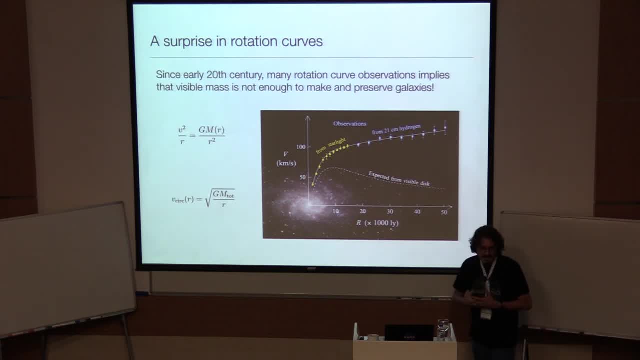 And divided by r squared. That's just simple Newtonian dynamics And just taking that Now, if you look at this at face value, the circular velocity then becomes: basically: it has to have a dependence of 1 over square root of r. 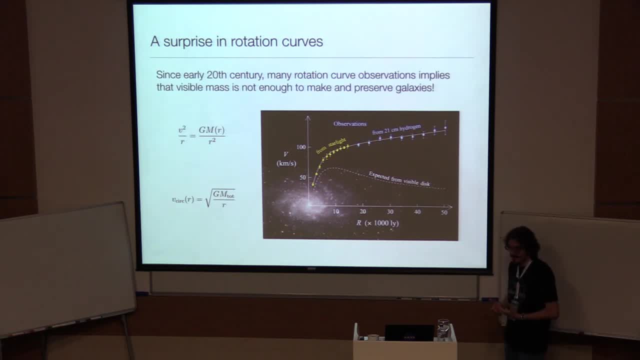 So, just starting from this theoretical expectation, people were expecting that when you collect such data, the circular velocity of stars, as a function of galactocentric radius, must decrease at least past certain degrees, And if you look at this, you see that it's very close. 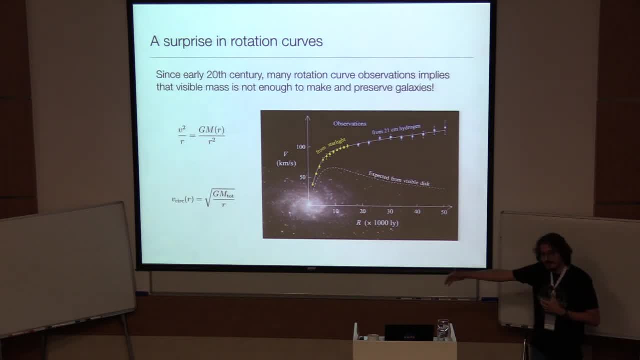 to the galactic center. Things are wonky So no one really knows what's happening, But at least very far from the galaxy, it has to be the fact that the circular velocities should fall off. I mean maybe not necessarily just 1 over square root of r. 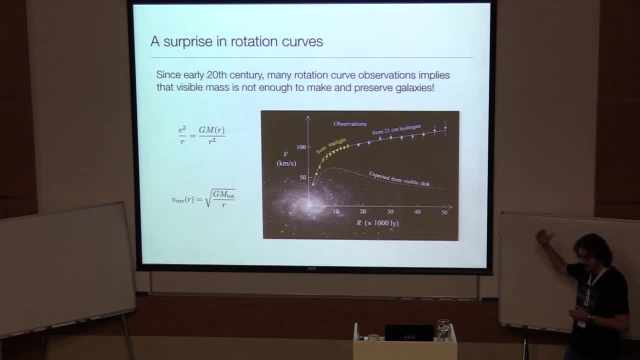 But at least it should fall off. But that was certainly not observed, And this first was observed for our own galaxy and then later for other galaxies, And this started to become known as the flat rotation curve problem- The fact that the expectation was wildly different. 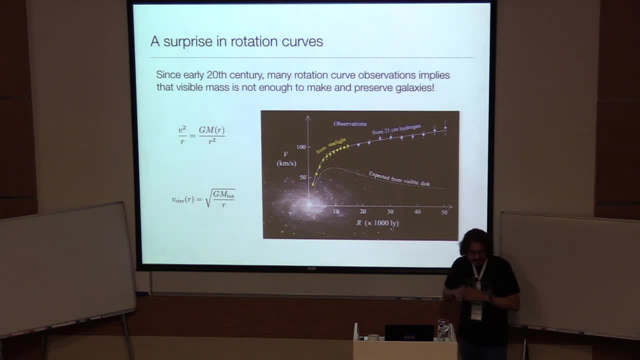 from observation about these rotation curves And obviously at this moment no one knew what was going on. People were wondering if there are other things that we cannot even see. In fact, this 21 centimeter hydrogen was a later addition into the game. 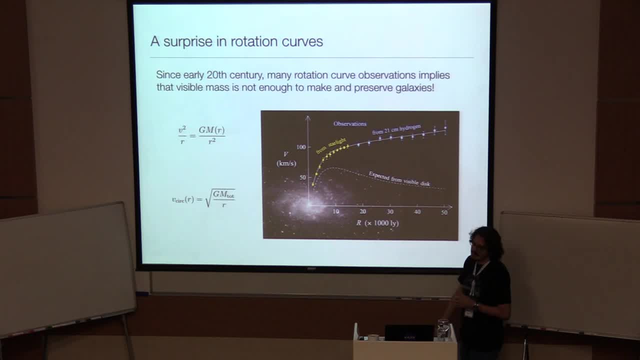 In the very beginning, people were only able to collect information from star And basically the rotation curve was the same as the rotation curve. And the way you do that is you collect spectroscopic data to figure out the line of sight velocity of stars. 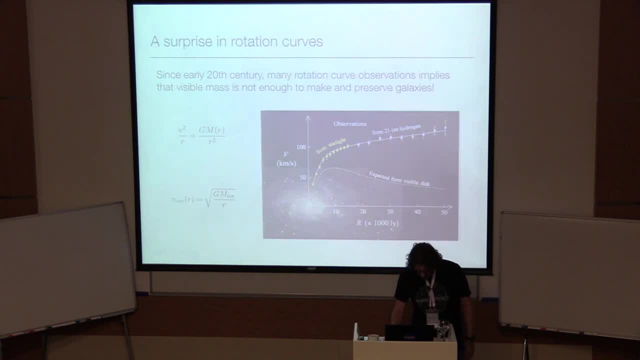 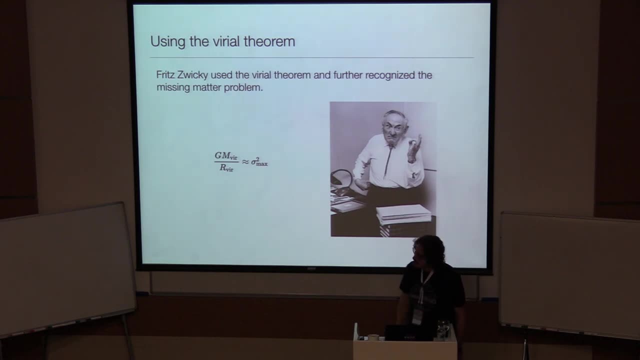 And that tells you, you can infer then, the circular velocity. Yes, please, Are we considering the effects of the gravitational effects of the things that we do see? I mean other, for example, if you consider a star that is orbiting around the center of the galaxy. what do you mean by so many things in between? What do you mean by so many things in between Other stars, planets and primordial black holes? Yes, So this certainly does include all the stars, So primordial black holes are basically just. we don't know if they exist, But I think you meant dead stars like actual black holes, that we know that they exist. They in mass budget. they're small, But certainly it has to be taken into account if you are going to do this. 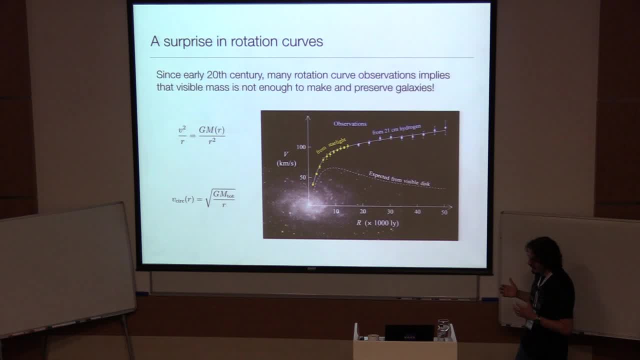 And later studies eventually started accounting for all of this. Now you mentioned a couple of them. I can mention more. There's actually dust that you have to take into account. There is obviously gas, So that has to be taken into account. 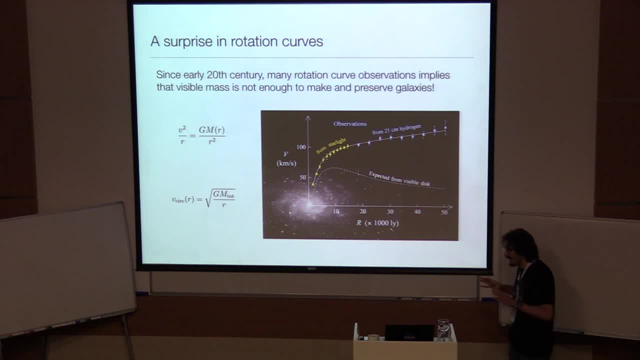 There is cosmic rays you also have to take into account. I'm not claiming that these, when you consider the mass budget, these are dominant, But still you want to take them into account. But and there might be, like rocks, like not necessarily black holes, 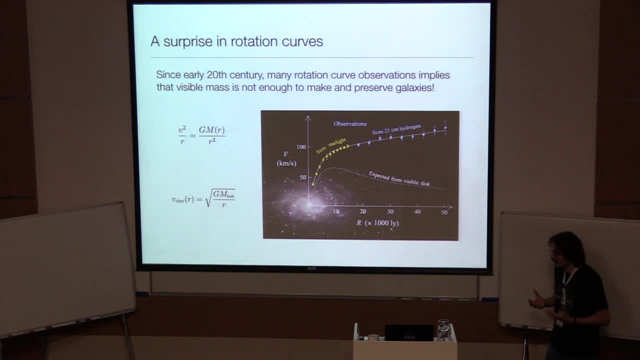 but things that just don't radiate much in optical waves but still are just baryonic matter that we know that they exist. People have wondered whether these could actually be the case And I will come to that during the talk. It just happens that they cannot make up. 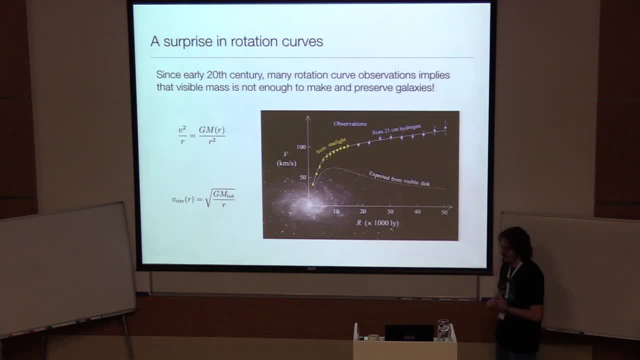 more than like 15% of this type of mass. They're called massive objects, compact objects, And they just can't make it. They are not enough. They're not enough. Yeah, They exist, but they are not enough. Any other questions on this plot? 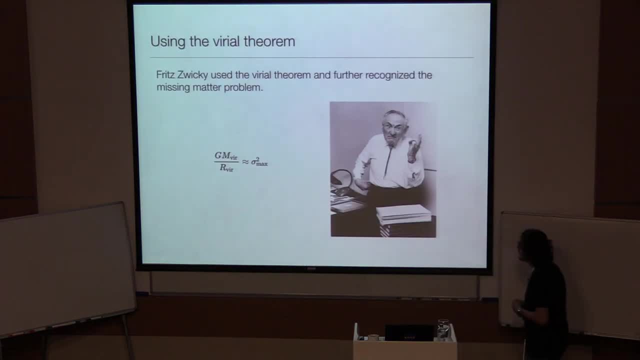 Crystal clear. OK, Well, things obviously evolve And there will be eventually more opportunities to ask questions too. So this was just the circular velocities of stars in our galaxy. But another thing you can do is you can use the Virial Theorem. 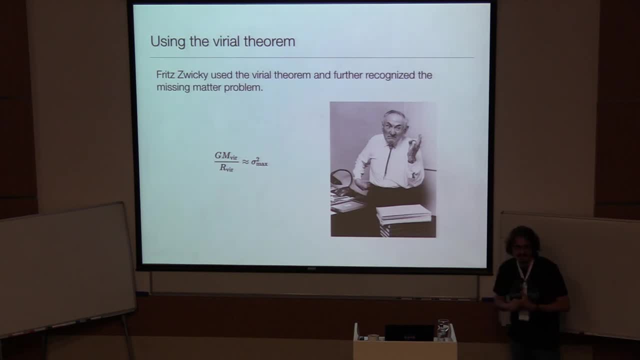 So I don't know how many of you are familiar with the idea, But Virial Theorem essentially allows you to extract information statistically from systems in which you just cannot solve analytically. Like if you have a two-body problem, you can just solve for the three-dimensional position. 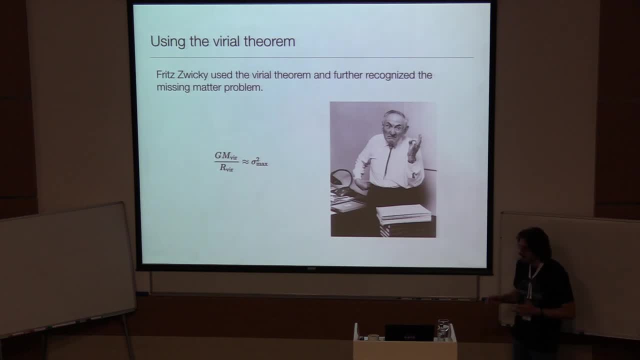 vector and the three-dimensional velocity vector of both objects. analytically That's fine. If you have three bodies, then you can just do some approximation. You can do it maybe. But if you have 10 bodies, 100 bodies, a million bodies, 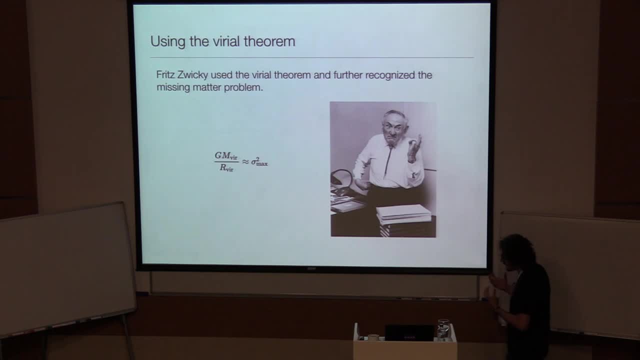 you just can't do that, So you have to rely on some statistical method to come up with a relation between the kinetic energy and the potential energy. And Virial Theorem is just that. It just simply says that if you have a bunch of particles, 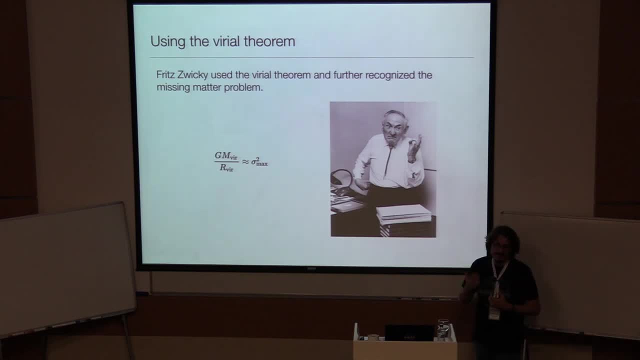 then the average kinetic energy is half the average potential energy in the system. So, using this, Pritz Zwicky, who's in the picture, who's making a funny sign, so he basically used the Virial Theorem to say: OK. 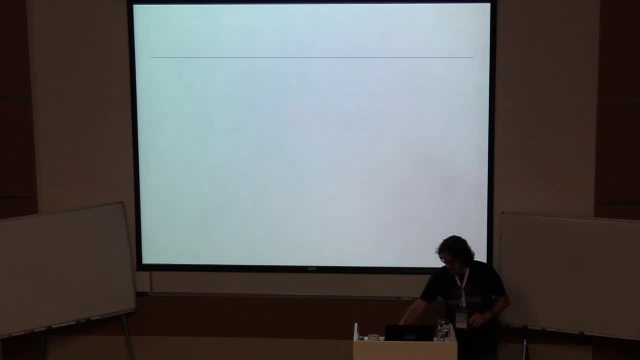 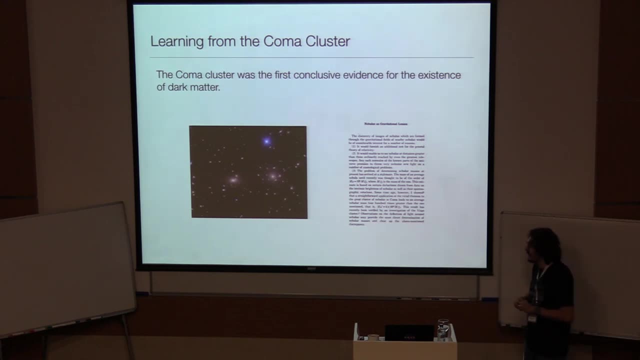 here's some cluster of galaxies And that cluster is actually going to be shown in the next slide. That's the coma cluster. So this is a bunch of galaxies sitting together, gravitationally bound. He basically did the same experiment, but now for galaxy. 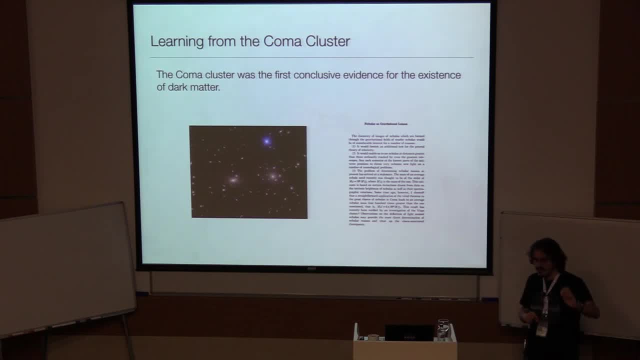 So he said, let me just measure the velocity. This is the dispersion of the galaxies. So that was an experimental challenge. but he did that And eventually he figured that the galaxies were moving at a velocity that is too much in order for this galaxy cluster to stay intact. 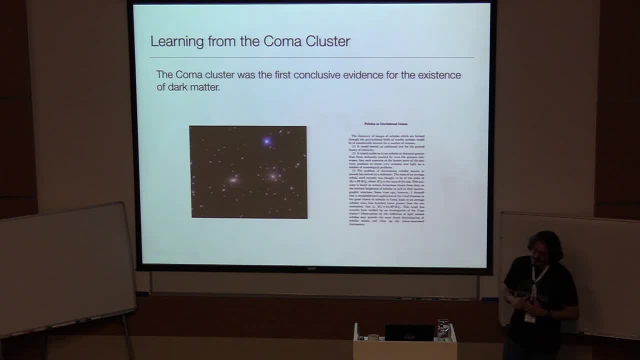 Now, another way to put this is: if you only had baryonic matter, that is, the matter that we know and love- in the standard model, then if you just start some simulation with the initial condition that these galaxies have whatever velocities that you measure, 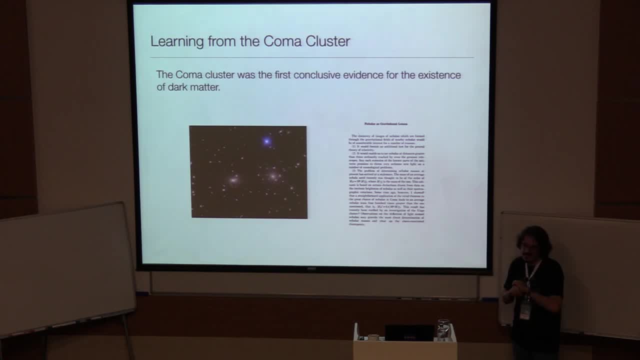 then if you run the simulation forward, the galaxy cluster will just fly apart. You just cannot preserve it. And that's the same essentially for the galaxy. Like going just back to this picture. if you start a simulation with the stellar velocities that you 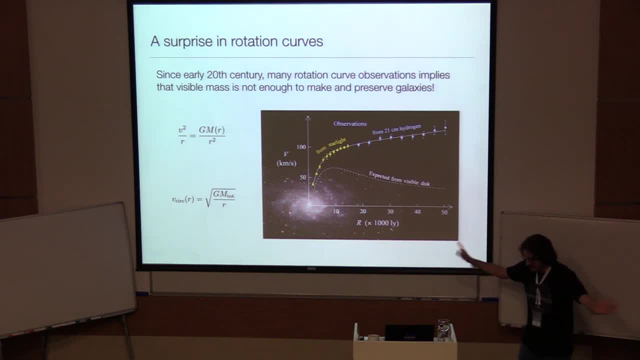 observe So without any dark matter, then the galaxy will just fly apart. You'll just not have any galaxy left in a few million years. Now this is a problem. Why? Because we make cosmological observations And obviously we use our sanity to say that galaxy, or in fact 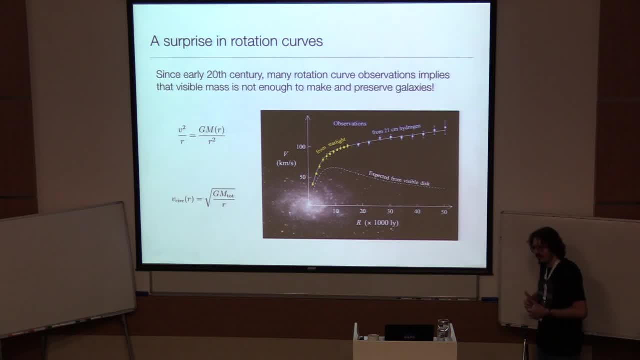 the universe. obviously it's evolving, That is true. But universe is quasi-stable, Like galaxies stay intact, because you can actually observe galaxies over billions of years And you make sure that they actually stay intact. So that's certainly against observations. 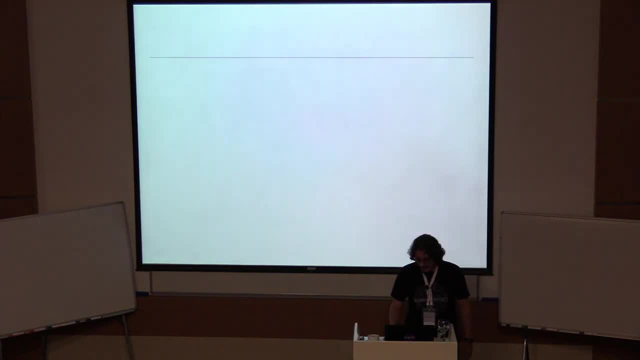 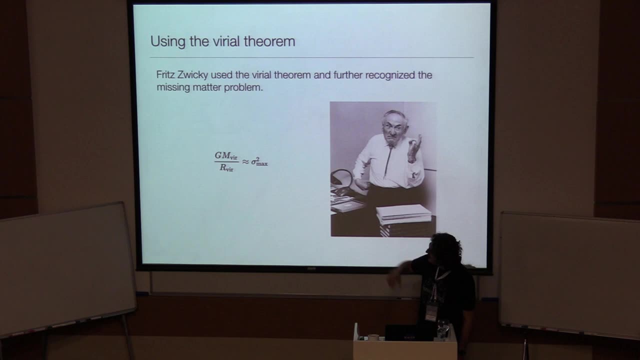 that the particles should just fly apart and you can't even make galaxies. And in order to make this conclusion, he used the video theorem where you just set, basically, the potential energy equal to the kinetic energy, which is proportional to the temperature and the velocity. 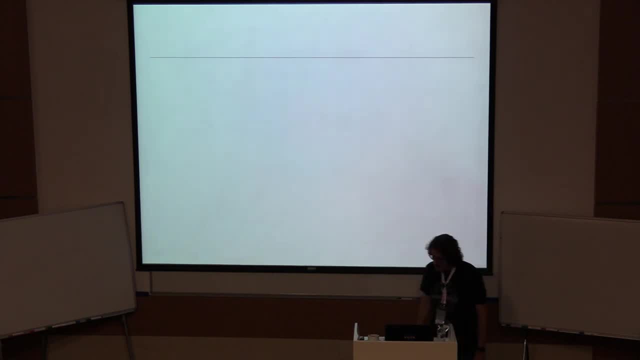 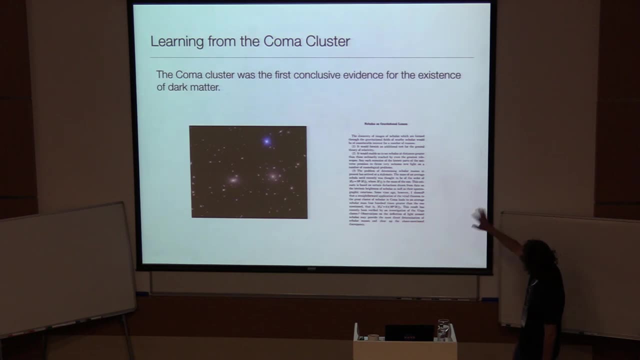 dispersion of the galaxies in the cluster. OK, So you can't really read, But on the right side I just put this. The context is really not important, But it just says nebulae as gravitational lenses. This is from one of Fritz Wiecki's work. 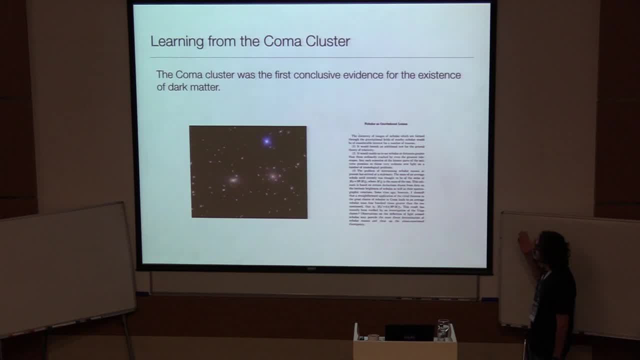 And it's just funny that at that time he was just calling these guys as nebulae And, more importantly, he actually makes a pointer to galaxy gravitational lenses, Because that's a really cool idea that he actually put forward, And I will discuss that in very much detail. 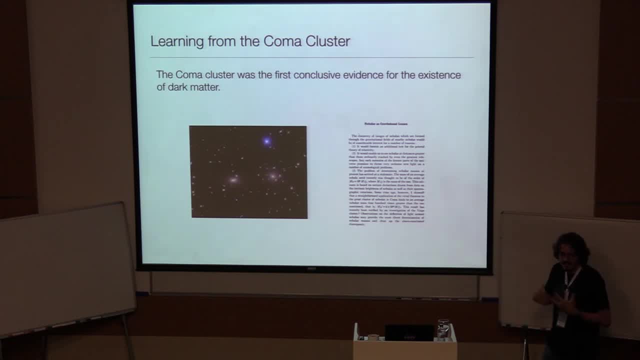 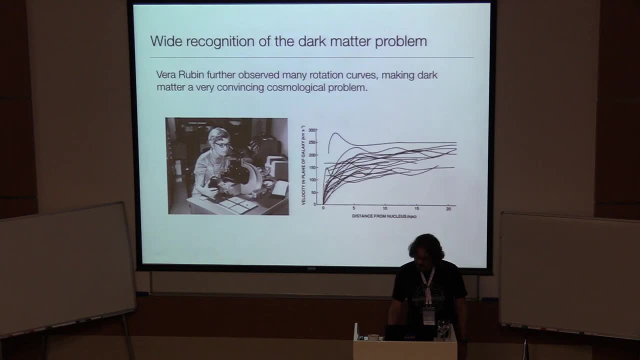 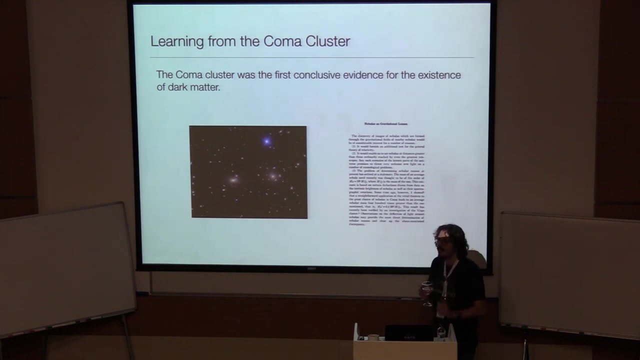 in the next lecture, using gravitational lenses to actually understand dark matter more. But that was a very futuristic idea back then. Excuse me, Yes, please. There's a wonderful story that I should know, Einstein in the original paper on gravitational lenses. 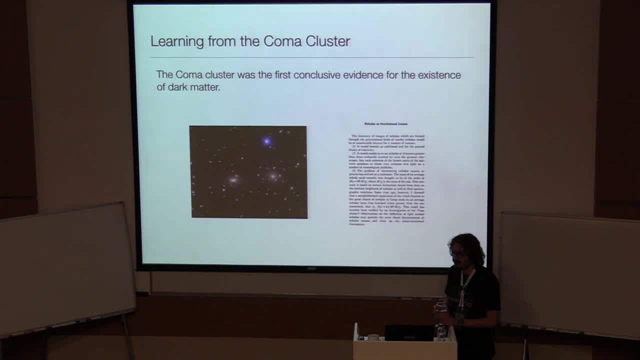 made an estimate and said that it was much too small to be ever true. Yes. And then he replied with a paper in Science whose content is basically: hey, Al, you didn't read my paper on the Kermit question. Yeah. 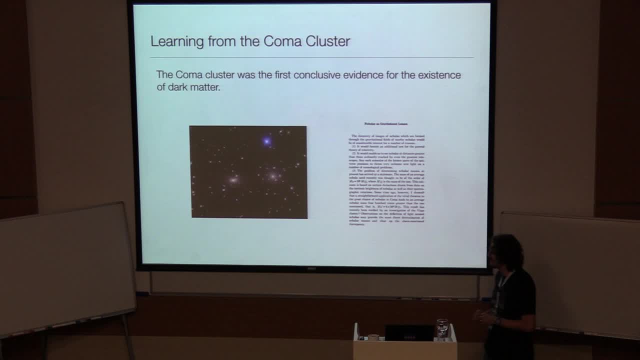 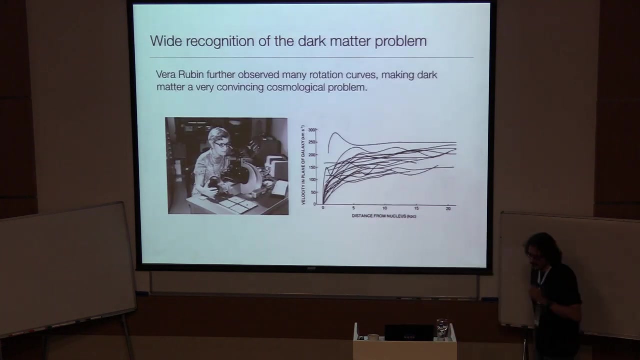 Yeah, Einstein had a lot of prejudices, unfortunately. Yeah, Yeah, thanks for that note. OK, any questions? so far, No, OK, So another very important figure where Ruben- I have to mention her name Because, first of all, she was a great scientist. 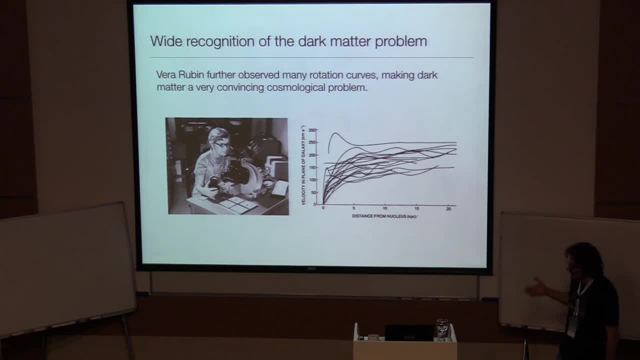 and certainly a leader for women in astronomy. But apart from that she was also leading the idea of dark matter in the sense that I've just shown you one rotation curve. But she and Ford working together, they basically published a paper, I think in 1980 or something. 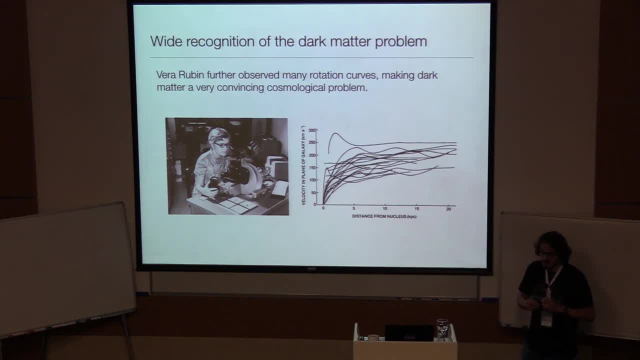 where they just nailed down the rotation curve, the flat rotation curve of many galaxies, And if you just stack them on top of each other, you get a figure like this, which is really cool. That just very, very clearly shows that rotation curves are. 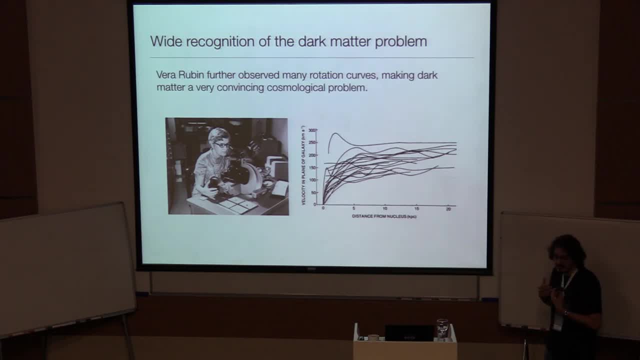 flat, or at least pseudoflat, They're certainly not decreasing and that there's a very, very serious problem, race cosmological problem, however you want to name it, But by then it was clearly named the dark matter problem. 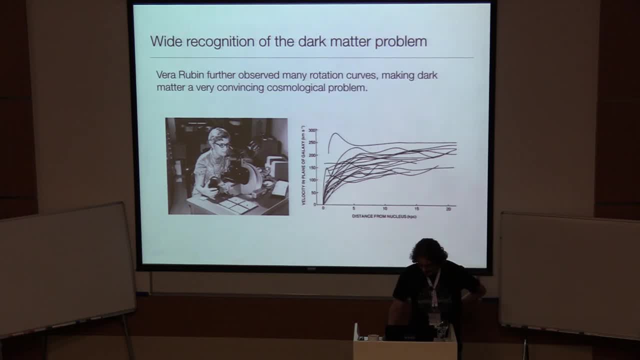 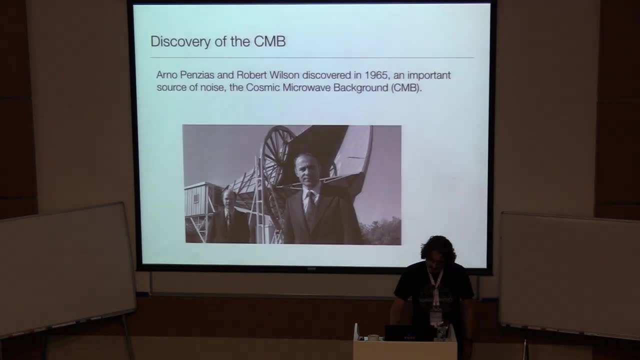 or the missing matter problem. if you really don't want to call it dark, Because it's certainly not dark, I will come to that, but it's got nothing with blackness. OK, so far, so good, And I'm a little slow, but it's fine. 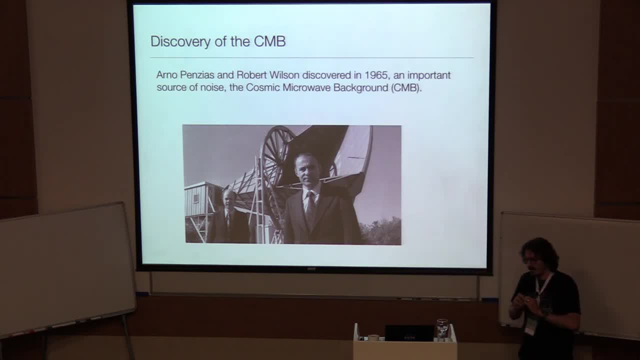 So I've discussed the rotation recurve problem. However, if you just take that as the only evidence for introducing a cosmological component, people might start laughing, Because unfortunately, in physics you need extraordinary evidence in order to postulate extraordinary theories. 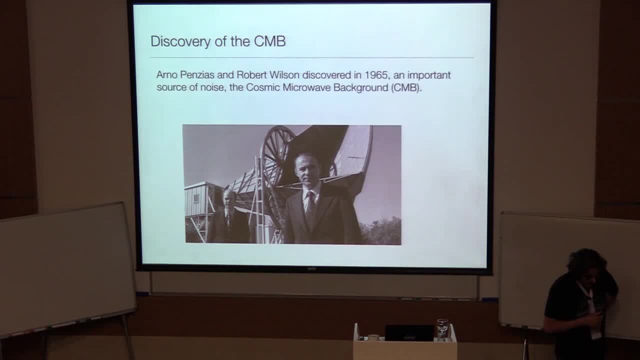 And dark matter is certainly an extraordinary theory. So if it was only the rotation curves, we probably wouldn't be believing in the existence of dark matter. However, the story is much more complicated, And I will just showcase a couple of examples from this story. 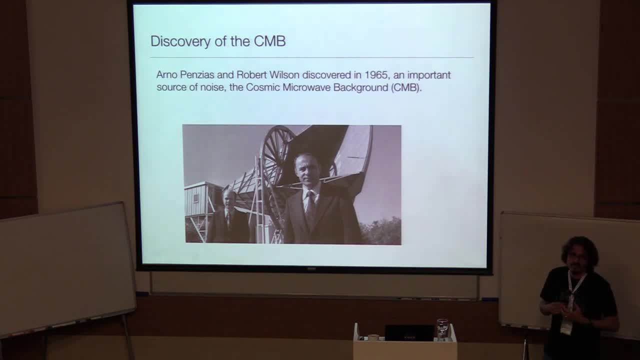 The very first one that deserves attention is the so-called cosmic microwave background. So in 1695, just by coincidence, two people called Arno Pentius and Robert Wilson discovered a source of noise. That's a funny term, but actually that's true. 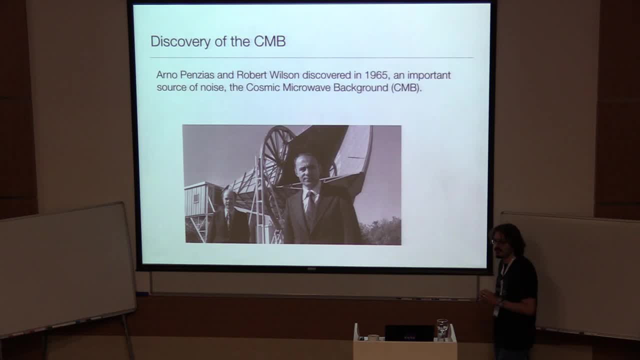 What they were looking for at that time was the neutral hydrogen emission from the galaxy. That was a very hot topic back then Because people were trying to understand the rotation curve of the galaxy and trying to make a map of the hydrogen emission. By the way, that hydrogen emission 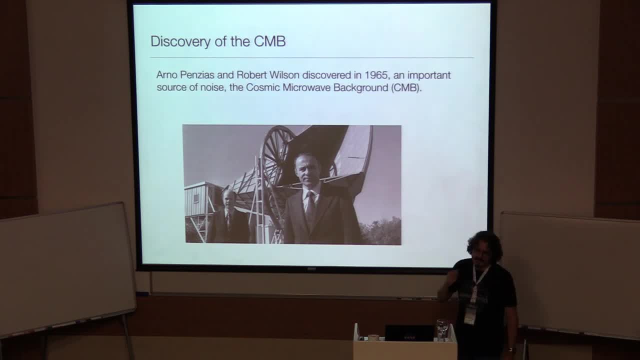 is the 21 centimeter emission which comes from the fine splitting of the two states. you probably know from quantum physics. So they were trying to look for that signal, And then they started to realize that there was a source of noise. However, they rotated their instrument. 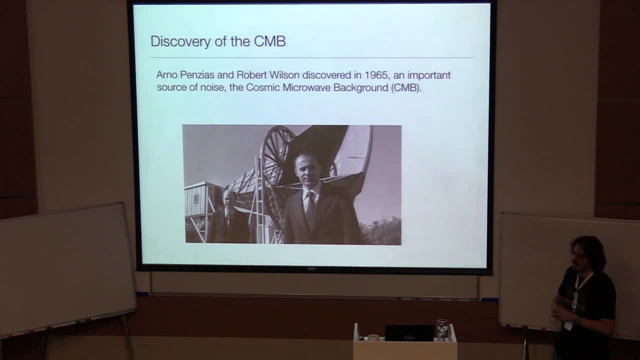 And wherever they were, they were looking for noise. Whenever they looked, they were just getting a constant noise, which was a nuisance, And they were just suspecting that it could have been the pigeons in the instrument or anything like that. They just did everything to remove the noise. 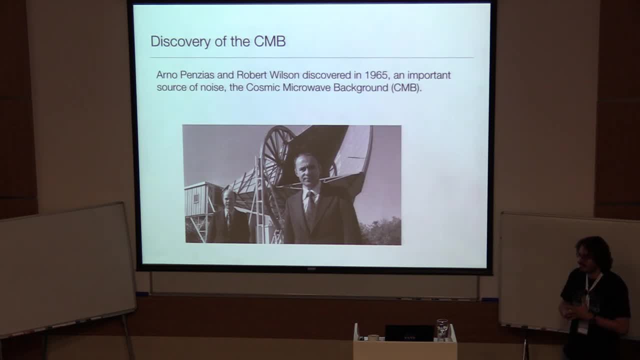 However, they failed And eventually they just made that leap of reasoning to say that there was actually a source out there, not even in our solar system, not in our galaxy, but actually extragalactic, And they called it the cosmic microwave background. 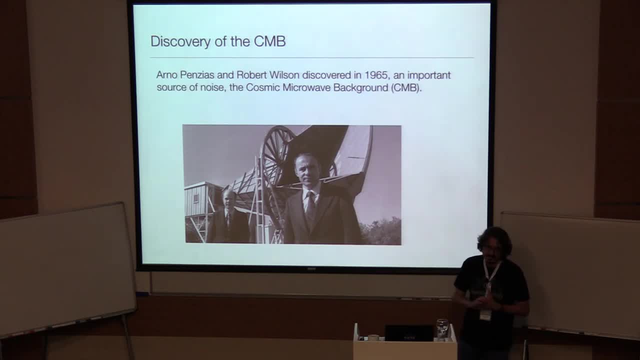 Cosmic in the sense that it sits in the cosmological context. It's certainly not galactic. It's extragalactic Microwave, because it's actually in hundreds of gigahertz. Well, it's got a thermal spectrum, which means that you cannot just give a particular wavelength. 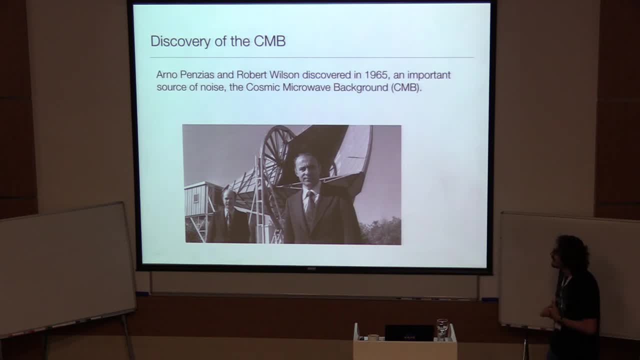 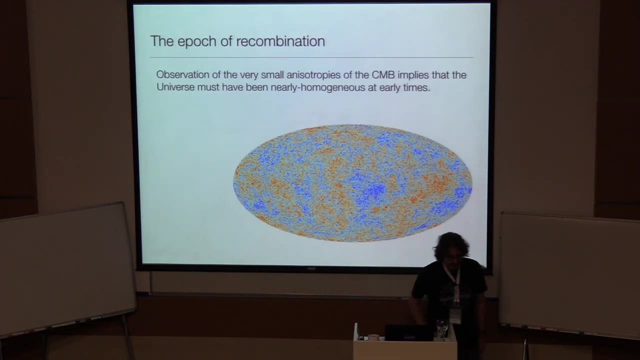 But it's got a thermal spectrum But it peaks at about 150 gigahertz And it's a background radiation, because it's at the background of pretty much anything that you hope to get using an extra instrument like this. So cosmic microwave background is a very, very important. 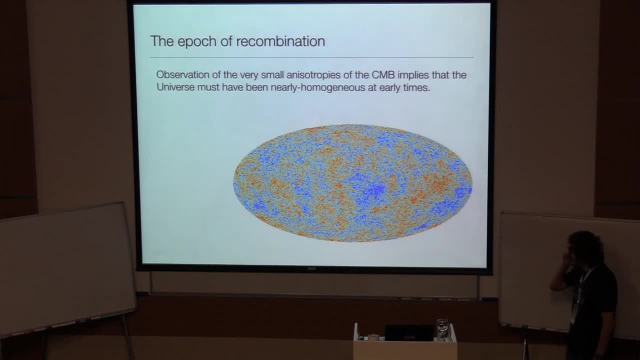 object for physicists and astronomers. So this is a picture, the full sky picture, of the CMB anisotropy. So I have to mention that. I was just saying that CMB basically is constant everywhere And that is certainly true. The reason I said that is because it's 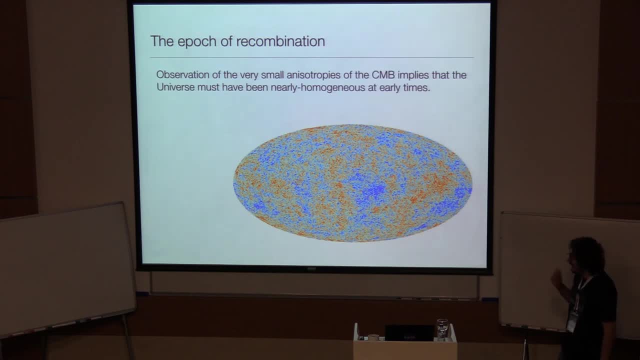 not galactic. It's not galactic. That is not technically true, but I did still say that just because the monopole term. if you just take a full sky map and decompose it in spherical harmonics and you can just 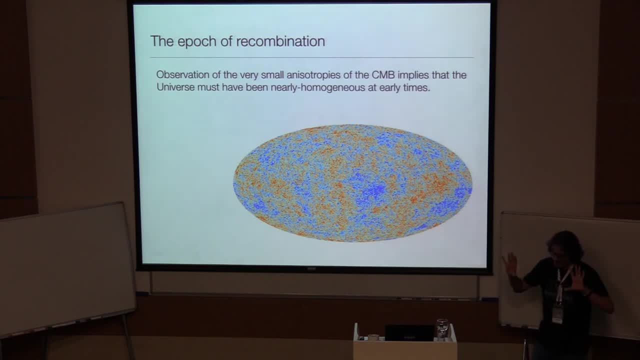 start talking about the monopole, the component that's just constant across the sky, or the dipole, which basically changes completely 180 degrees away. So those two terms are really important. The monopole term is extremely larger compared to whatever other higher terms you might have. 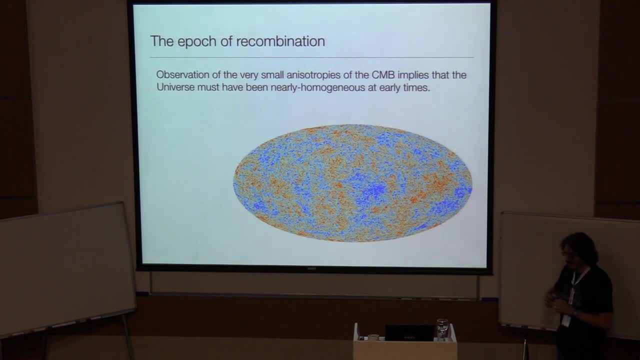 from that spherical harmonic decomposition. So because that is so large, we say that CMB is constant across the sky. Certainly that is not true because of two reasons. First, there is the dipole term and that is not a cosmological thing. 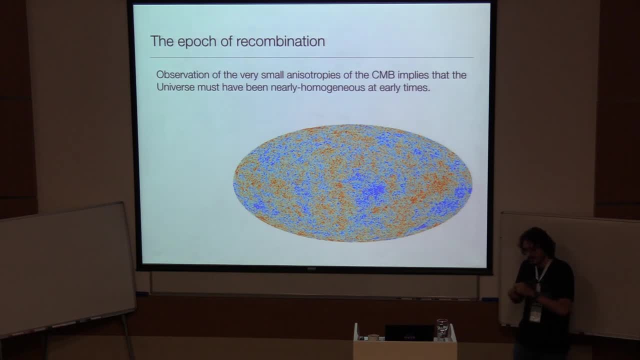 That is just because our local group is in motion. with respect to the CMB, It is a cosmic microwave background- And also because our earth, for example, has some rotation around the stars. Our star has a rotation about the galaxy, etcetera. 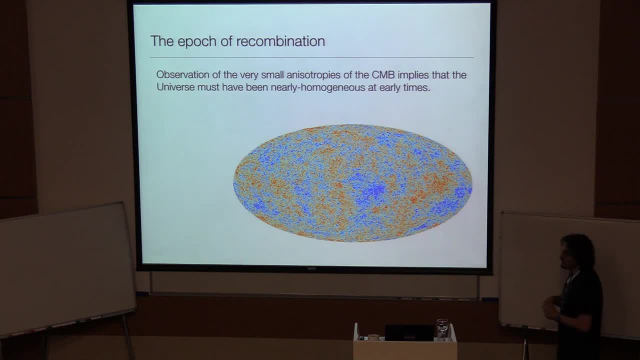 There are other types of motions as well. But second, there is actually primordial anisotropies in the CMB, not related to our motion in the universe, And that part is really really important, pristine information. So that's the part that's the most important. 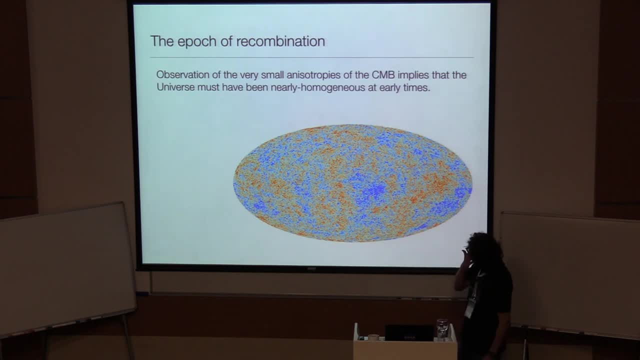 that will teach us about dark matter. Now, so far, so good. the takeaway message from this slide is that the initial conditions to the universe must have been really, really homogeneous, And I haven't really made that connection yet, so I should probably make that before making this statement. 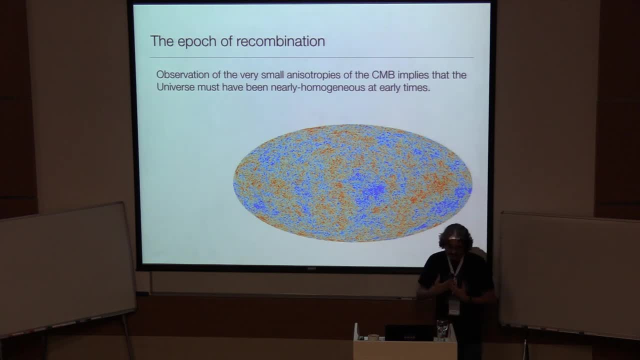 So cosmic microwave background radiation is a radiation that we think is coming from the Big Bang, the beginning of time. Obviously, I don't really mean t is equal to 0, but I actually mean t is equal to about 400,000 years. 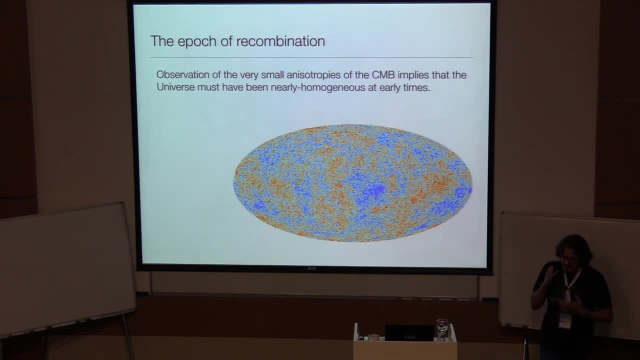 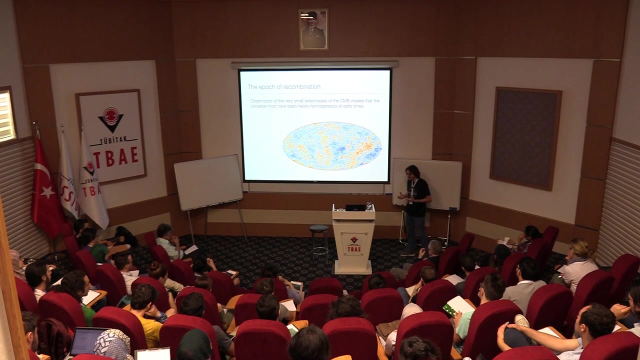 And back then what was really happening was basically, if you just think about the universe at its very early stages, the universe is pretty hot and dense and has a really high pressure in the very beginning And then, as the universe expands, the pressure goes down, the temperature goes down. 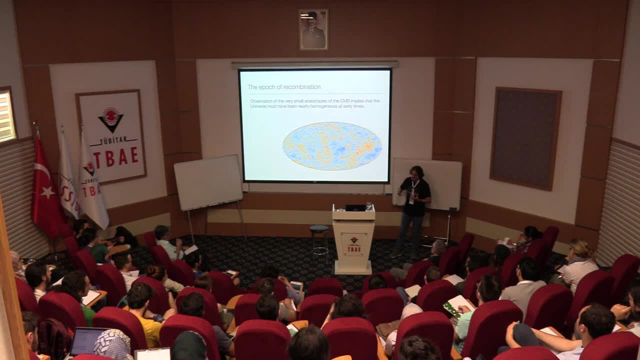 And when the temperature goes down, temperature just means energy, Average kinetic energy per molecule. So eventually there happens to be a time in which the mean kinetic energy of the constituents, which are essentially electrons and protons, becomes lower than the binding energy of the hydrogen atom. 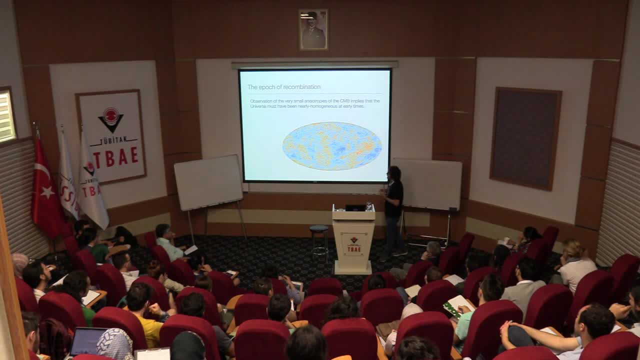 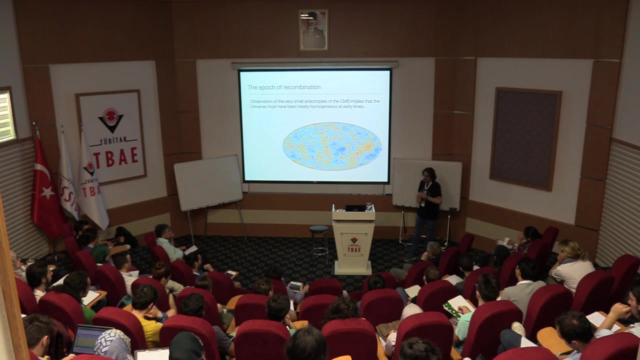 Once that happens, we call that recombination. The electron and the proton recombines to form neutral hydrogen atom, And once that happens, a very special moment in the history of the universe takes place, simply because the photons that used to be just scattering all around. just because the electrons and protons are charged, particles suddenly are let free at the time of the recombination, Because after the recombination you have neutral hydrogen Whereas before recombination you have charged particles. So photons suddenly have a much higher mean free path. 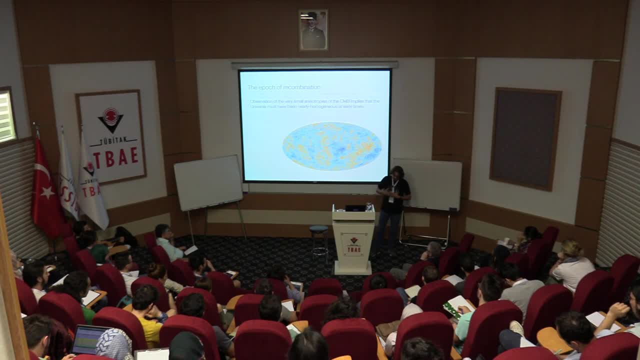 than before, And that's essentially the result. That is why we tend to observe these photons from this last scattering surface about 400,000 years after the Big Bang, Pretty much unimpeded. I mean, the mean free path of the CMB photons is really large. 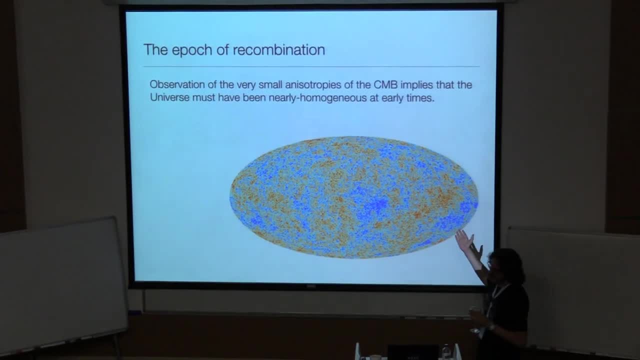 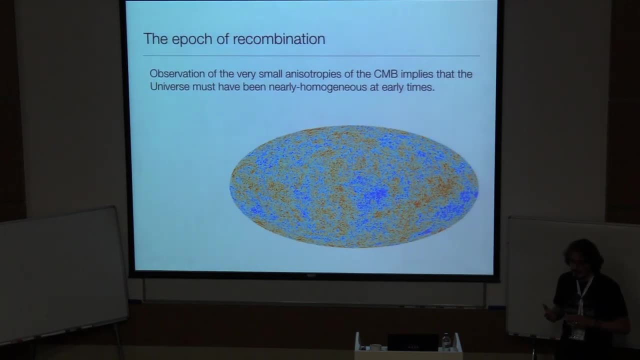 Yes, Yes, thanks for the note. So this picture basically only shows the terms that are higher than the dipole, And that essentially, is important, because if I were to show the monopole it would be a very boring picture. 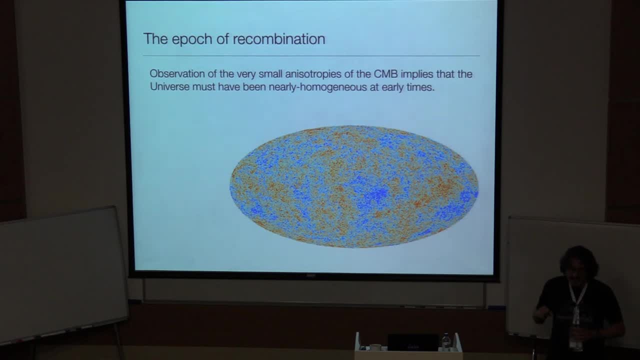 It would just be a single color, without any information, If I were to show you the dipole, which is about millikelvin. So, by the way, I didn't give the numbers, But the monopole is 2.7 kelvin. 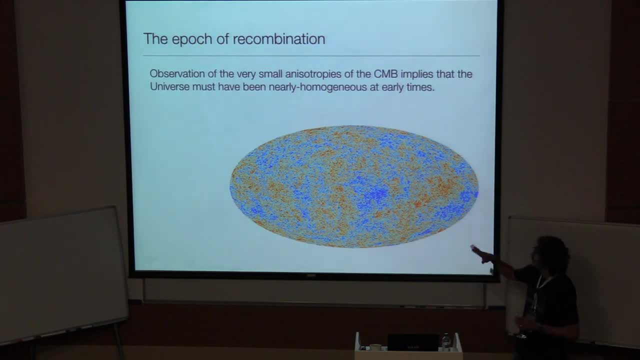 The dipole is about a millikelvin And the dipole is about a millikelvin. So if I were to show you the dipole, the dipole would just be like a very smooth picture with two poles. But if you just remove those two, 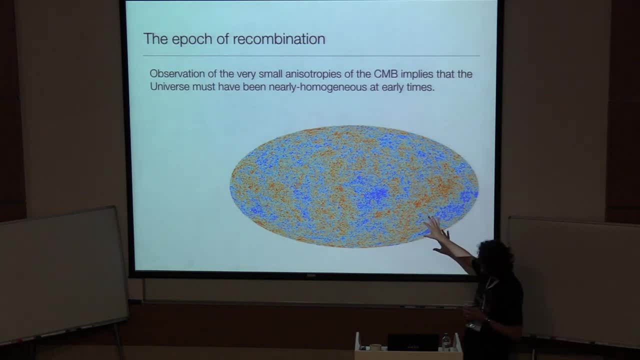 then you get this type of picture. There are certain features. The most obvious feature is a degree size feature, which I will come to at the very end of the talk when I talk about baryonic acoustic oscillations. But that's a result of this propagation of pressure waves. 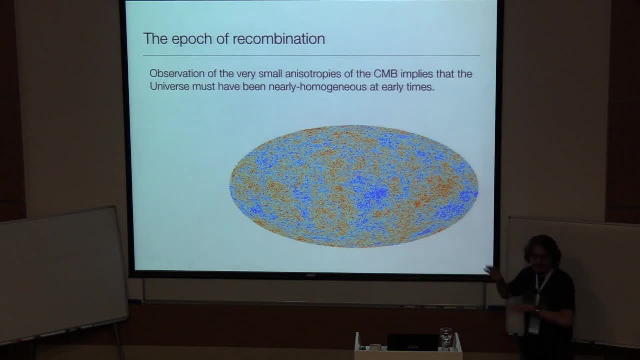 We will come to that, But essentially you see fluctuations of all scales. So these are actually cosmological and very, very interesting. Yes, please, What if there is a primordial dipole in the scene? You said that we remove the dipole. 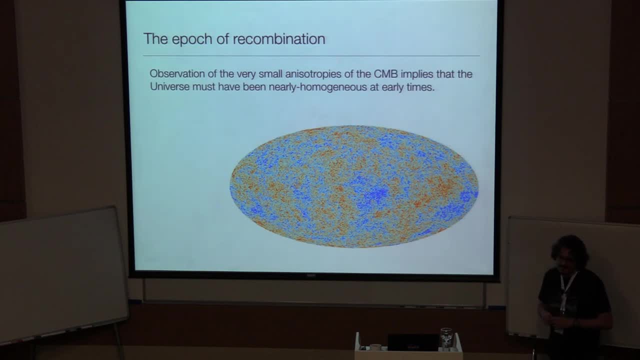 Yes. So removing the dipole obviously makes the assumption that all the dipole is due to the motion And they are degenerate. So we would have no hope of finding if there was a dipole that is cosmological. That is simply not possible. 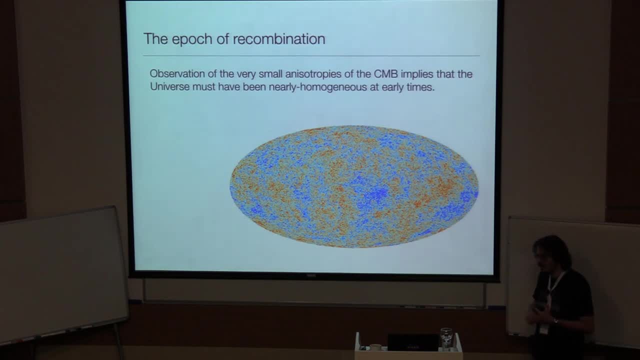 I mean they're completely degenerate. What you can do is you can study the fourth or the eighth order multipoles, like the octapole and the quadrapole. They start containing some cosmological information. For example, one thing that may catch your eye: 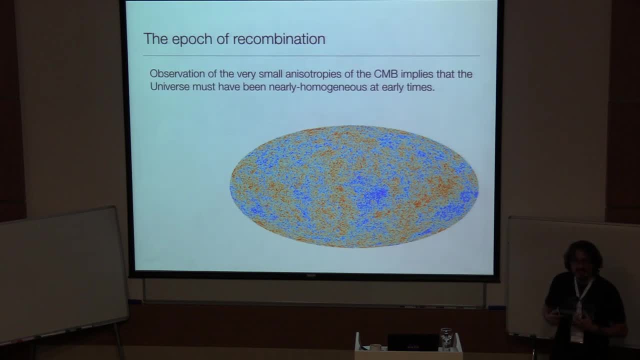 is this cold spot here? Things like that. you may see, maybe there was some process pre the inflation that caused this and people have wondered about that. But the problem with that is we have only a couple of such modes and we have a really 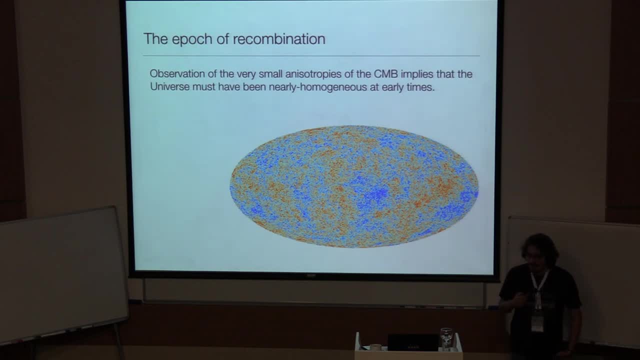 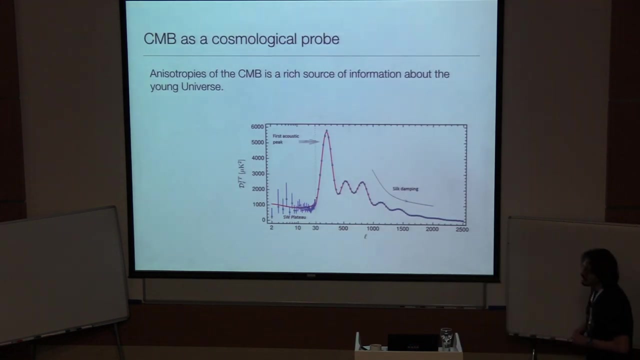 large cosmic variance. So no one really can say for sure that they point to a particular physical process before the Big Bang. But you can only speculate and unfortunately we have only one universe to observe Other questions. OK, So if you take that map and do the spherical harmonic decomposition that I was just talking, 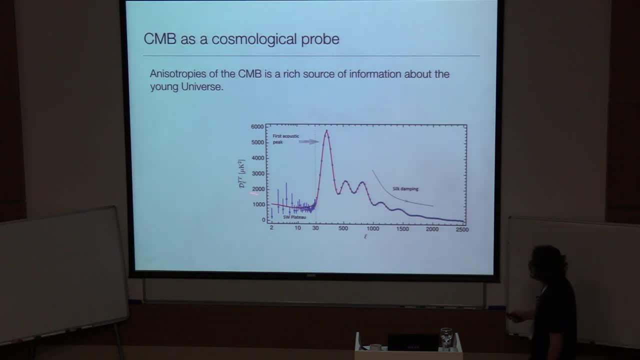 about you get basically this picture. This picture tells you the power spectrum of the CMB, the cosmic microwave background, The power spectrum. essentially this is rescaled, so it basically tells you the power in every frequency. So this L is the spherical harmonic component, so it's in the frequency domain rather than 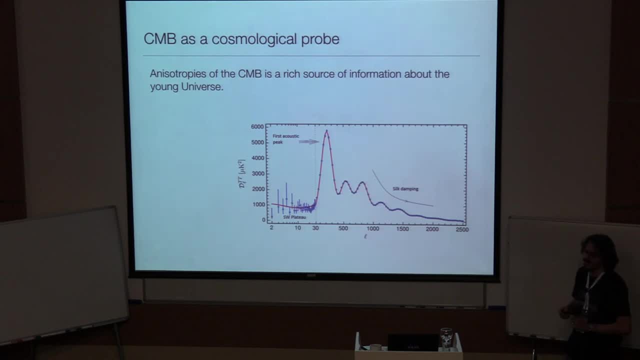 the position domain. So in every frequency bin it tells you how much power there is. So if you basically sum up all the y values here and multiply by the bin width, then you basically start getting the. obviously this is a discrete one. I'm giving the analogy. 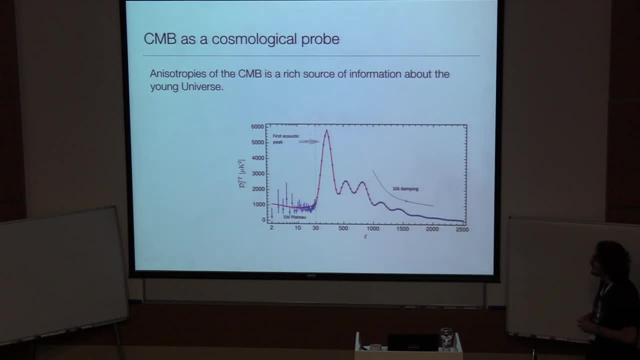 here You basically get the full variance of the CMB. This is just breaking down the variance into components, And so this power essentially contains a lot of information about the initial conditions of the universe. I won't go very much into detail because the idea is to discuss dark matter here. 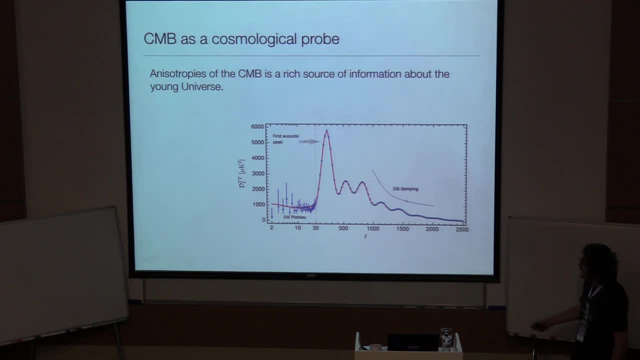 So there's a lot to talk about. One could give like a 10-hour lecture on just one plot here. It's really rich physics. But I will only just mention that This very first acoustic peak here wouldn't just be there if we did not have dark matter. 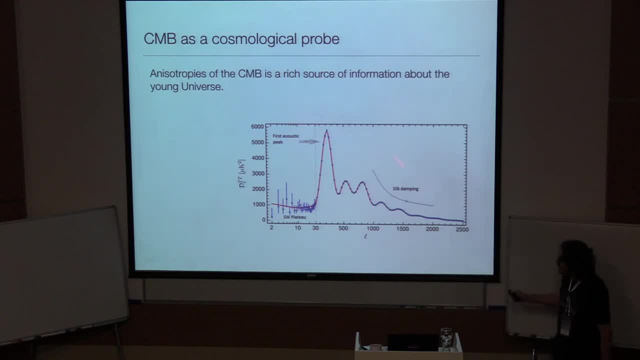 And well, if we did not have dark matter, this would just look wildly different. not just the acoustic peaks, But the thing that would get affected most if we did not have dark matter would be these acoustic peaks And just putting it in layman terms, the reason is dark matter particles. I think I have a 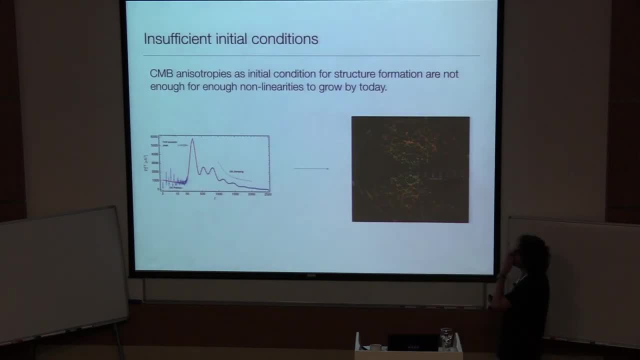 plot on that. No, I don't, Sorry. OK, That will come later, But I'll just state it in words. Dark matter: doesn't we think that dark matter doesn't interact electromagnetically with the rest of the cosmic plasma? 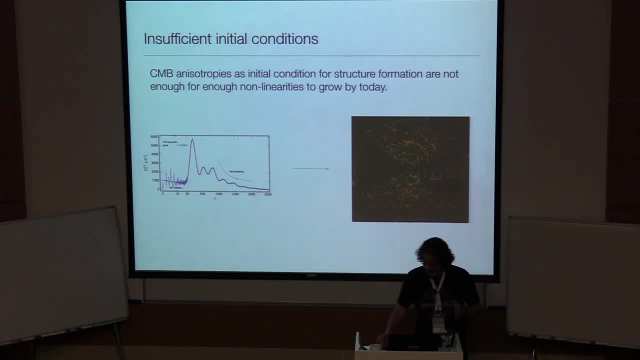 That means prior to recombination. when the baryonic matter, that is, the electrons, the protons and various other particles that you know, are tightly coupled to the photons, just because they are tightly coupled to a radiation plant, The radiation field, they the density perturbations, the contrast, the density contrast in them. cannot grow much. It just grows so slowly it's stalled. basically, However, dark matter, not being coupled to the rest of the guys in the cosmic plasma, is freely able to just grow its structure prior to the epoch of recombination. That is the key point here. 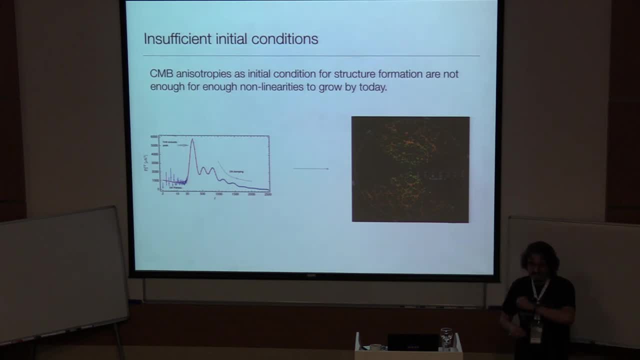 Because dark matter. if dark matter exists and is decoupled from the rest of the cosmic plasma, it actually contains a lot of structure that is not visible in the baryonic matter. Now why is that important? Well, the idea is the following. 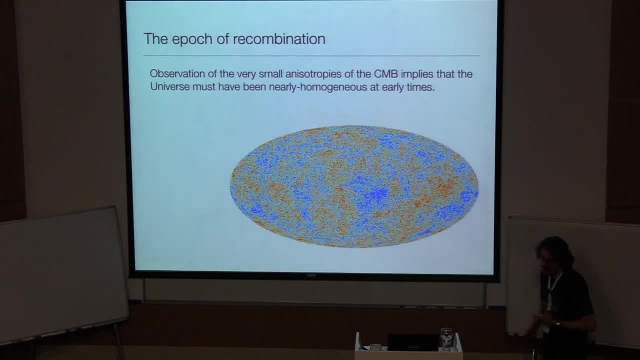 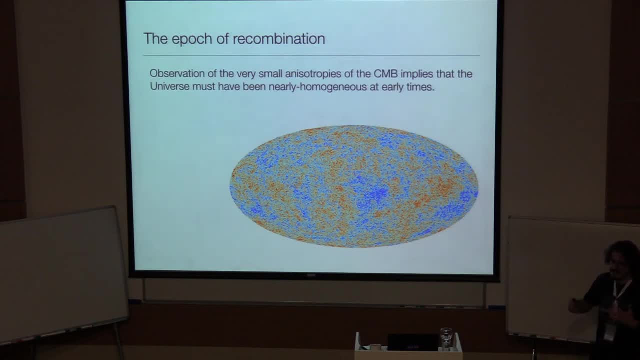 today in the universe, All these galaxies and stars and planets, et cetera. We cannot produce them. The only way to produce them is to have edifices. The only way to produce them is to have additional structure at the time of the recombination. 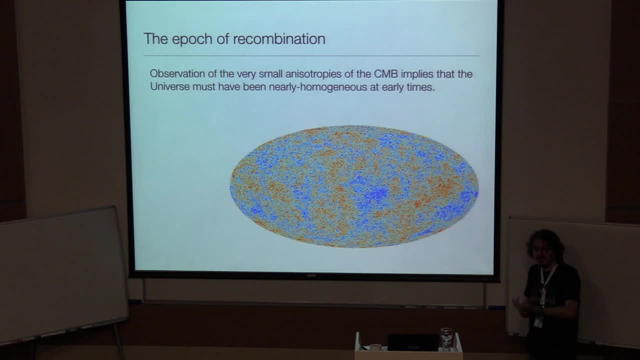 And in order to produce that, you postulate the existence of an additional component called the dark matter, that basically starts growing its structure prior to the epoch of recombination. So you see the idea: There is an additional component that must exist in order for our universe to grow enough. 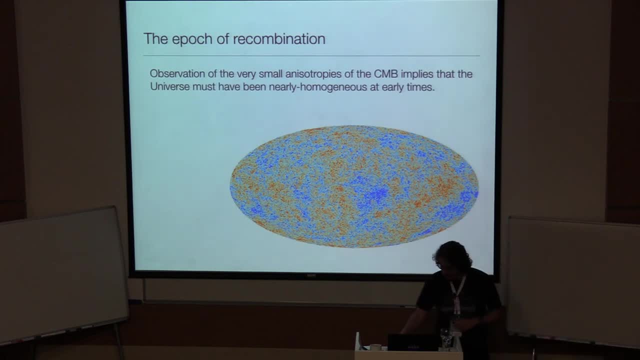 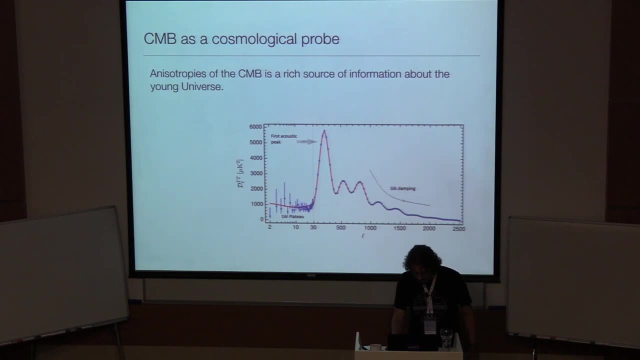 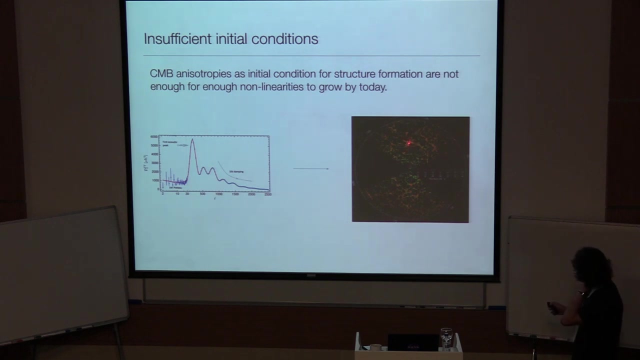 structure by today. That's the key point And hopefully it will become more clear towards the end of the lecture. So this is more like an introduction. So here you see a picture of the large-scale structure of the universe. So these guys basically are called filaments. 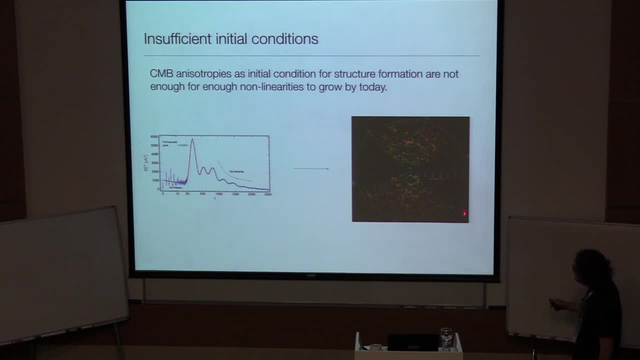 And so basically, the scale of this contains pretty much the observed universe. It's like looking at the universe from above- Well, only literally, I don't mean it, But just laying out all All the known galaxies. This data basically comes from spectroscopic surveys. 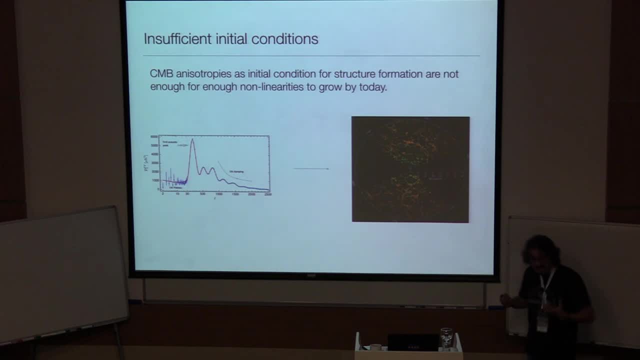 And it just tells us that there's a lot of structure, Not just at our scales, like stars, planets, et cetera, but also at the very large scales. In order to produce those very large-scale structures, you have to start structure formation. 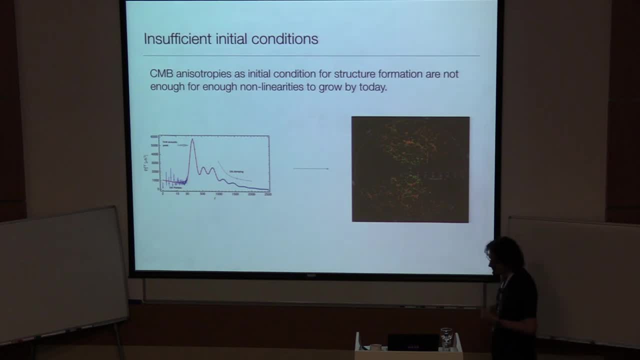 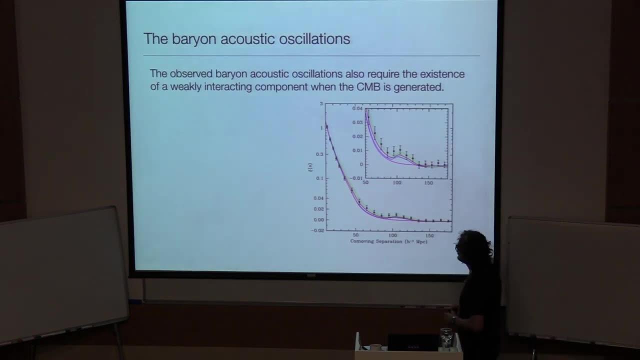 very early, And the only way to do that is to propose the existence of dark matter. OK, Thank you. OK, So another point about baryonic acoustic oscillations. So I've already talked about the fact that there are certain sound waves in the universe. 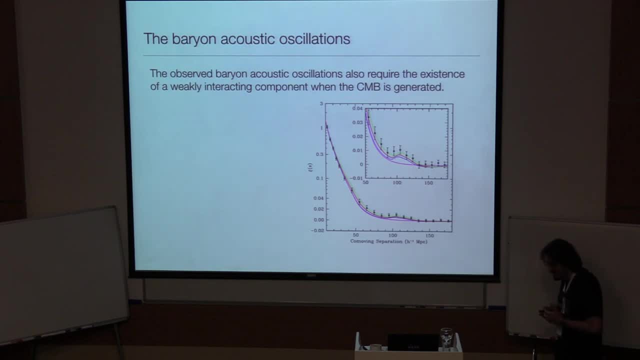 prior to the recombination And those sound waves basically propagate at a particular speed And by the time of the recombination it reaches a particular distance. In co-moving coordinates that distance is about 100 megaparsecs. roughly, very roughly. 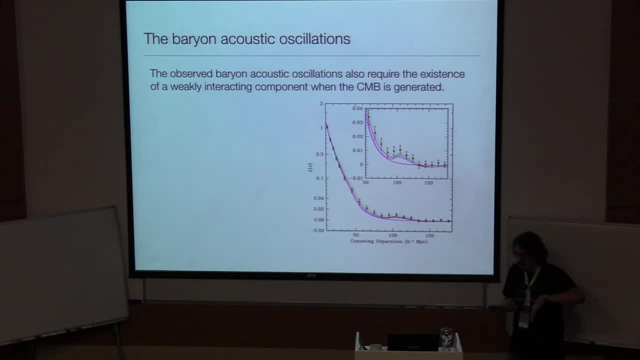 And basically, if you make a plot of the two-point correlation function of all the galaxies in the universe- basically just look for correlations- then you actually get a bump at about 100 megaparsecs. That's one of the coolest results in cosmology. 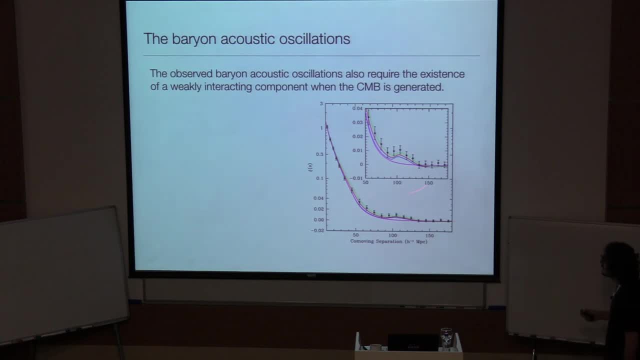 It's a result by Daniel Eisenstein, who was in my thesis advising committee, And he basically has led this effort And it had basically many generations. Currently There's the fourth generation experiment trying to reconfirm this and make it even measure. measure it even finer. 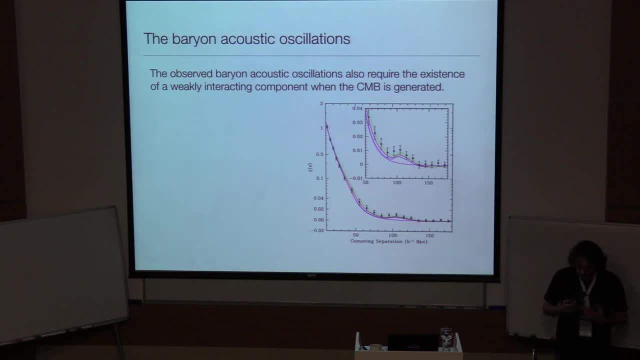 And this bump basically allows one to infer a lot about the pre-recombination physics or universe, Because it tells you very, very precisely the speed of the sound in the cosmic plasma And it tells you how much radiation there is, how much dark matter there is. 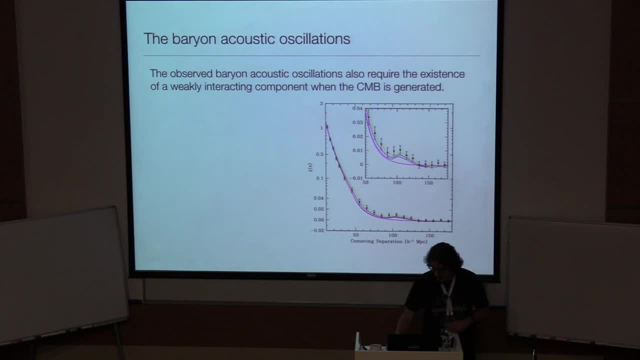 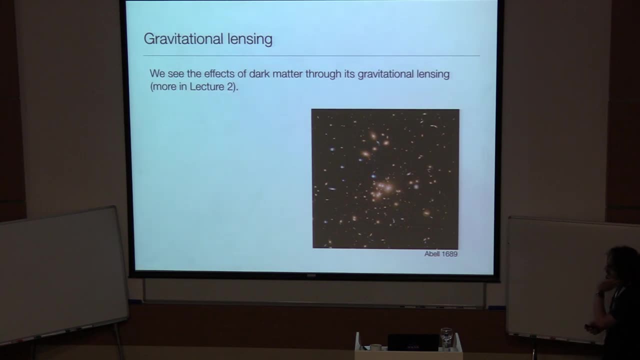 So along these lines, all the dynamics of the fluid in the cosmic plasma. OK, So now we will switch gears again. I'm done with this CMB part of the evidence. but the list of possible evidence that you could count for dark matter actually is pretty long. 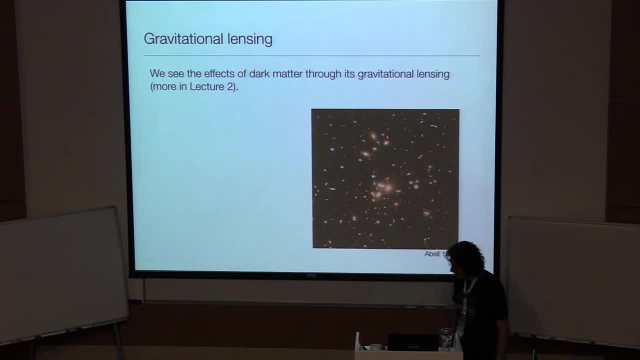 So I will only showcase some of them. as I said, Another evidence actually comes from so-called gravitational lensing, etc. … etc. into much detail about this, because it is the main topic of my next lecture. 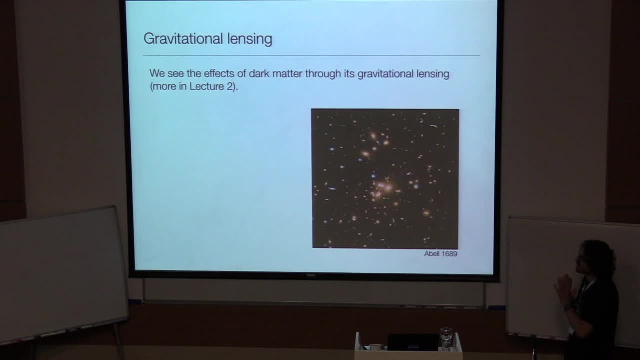 That's why let me not spend too much time on it, other than saying that gravitational lensing essentially wouldn't happen the way it does if we did not have dark matter. And without actually defining what gravitational lensing is, that statement actually is very, very futile. 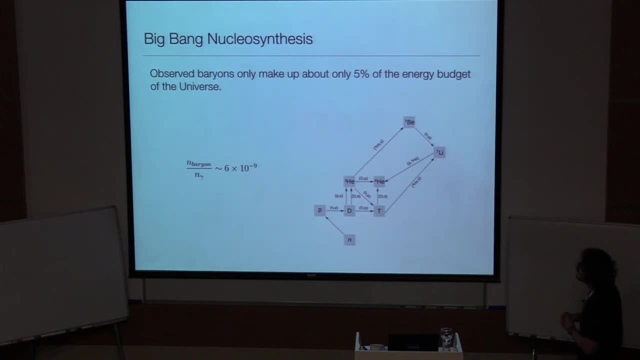 But you get the idea. So we will discuss that in detail later. So I don't want to steal away second lecture's material. OK, So another piece of evidence we have is from the Big Bang nucleosynthesis, By just looking at certain stars that are not very evolved. 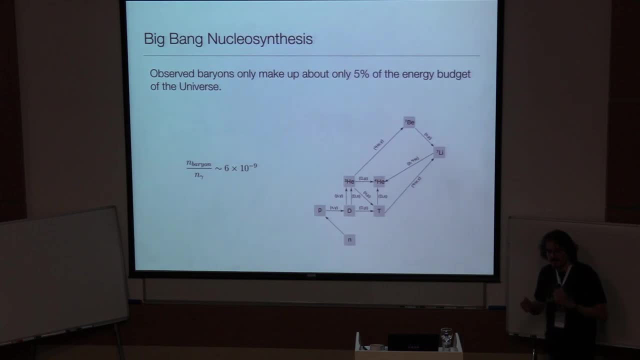 you can start figuring out the ratios of the primordial elements, the elemental abundances, And that tells you roughly the baryon to photon ratio in the universe, or rather the average baryon density or the amount of baryon there is in the universe. 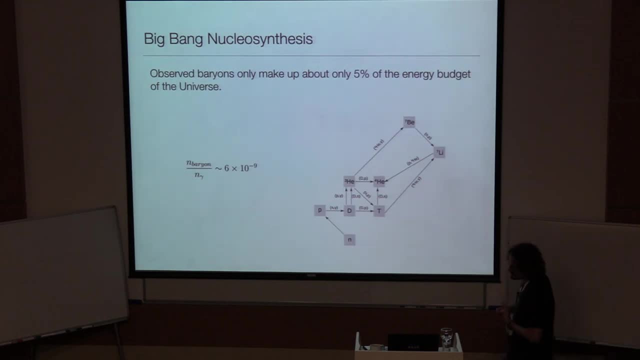 as a function of the energy content of the universe, And that number is about 5%, very roughly, And although it's not a very precise number, I think the mean value tells you something about it. That is, we only can see electromagnetically. 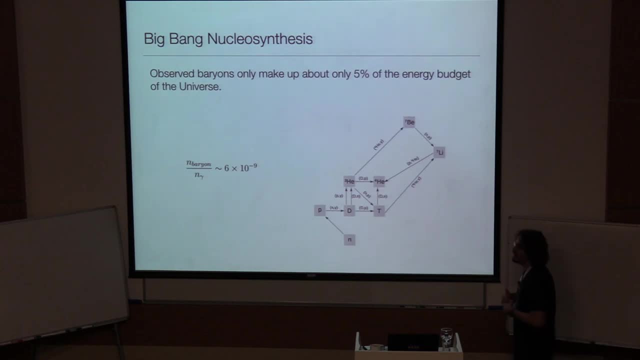 5% of the universe. The rest is dark matter. And yet another point, OK, OK, So another component that I haven't even mentioned and won't really mention in these lectures: the so-called dark energy. they basically together make up the concordance model of cosmology. 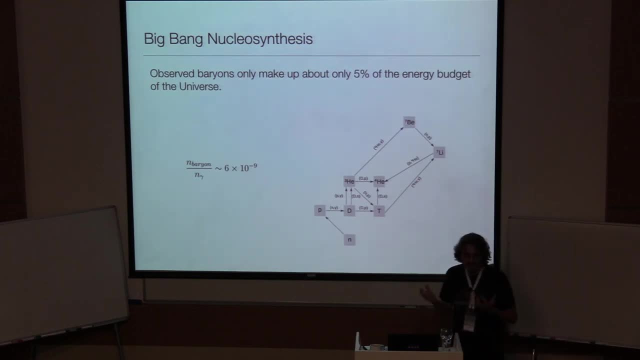 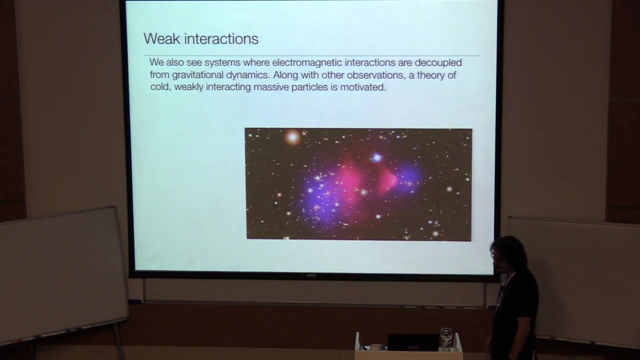 But the idea here is that there is yet additional evidence, apart from the CMB, apart from rotation curves, that if you just start counting baryons in the universe, they just can't make up for the full energy budget of the universe. 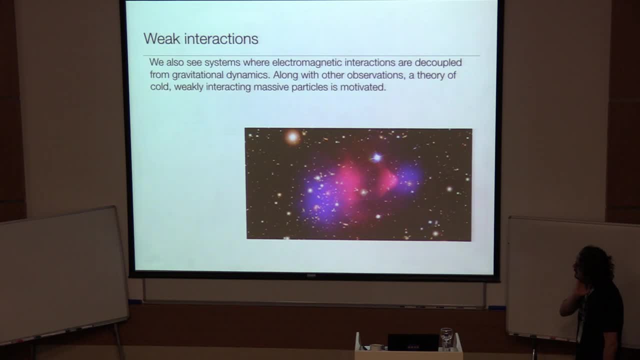 OK, So yet another evidence I think that's worth noting is our systems, in which you see a collusion, let's say, between galaxy clusters, But at the end of the collusion you figure out that some content of the galaxy clusters are essentially not impeded by this collusion. 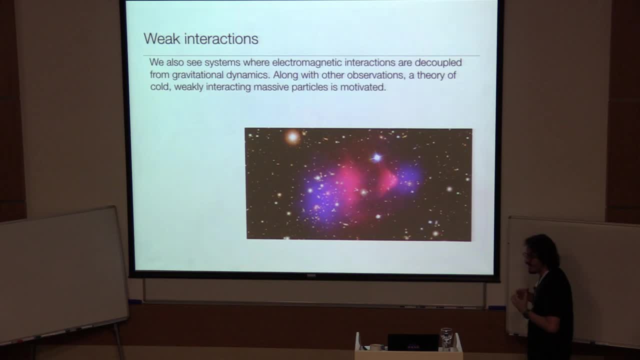 And the baryonic component that you see is actually impeded or is subject to friction or collusion. So this plot basically shows the collusion of two clusters. It's called- you probably know the name- it's called the bullet cluster. So what's happening here is you have two clusters. 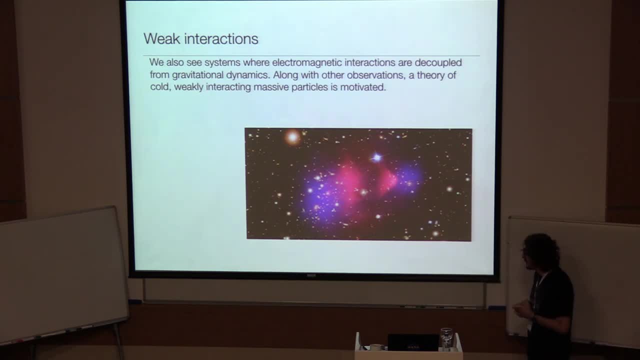 And the clusters obviously have a lot of hot gas in them, the intercluster medium. So the red color is showing basically the visible the hot gas. that's basically very hot, just because it just collided with the other cluster. But you can see that it's got the shape, that it's almost 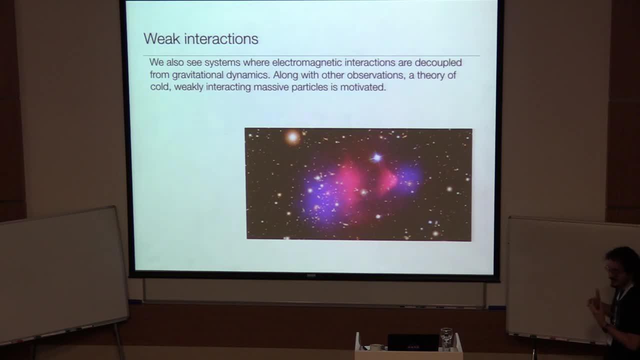 like, went through the other cluster as a result of the collusion. Now wondering about the blue? the blue part is actually not a direct electromagnetic measurement. You don't just measure the gravitational field. What you do is you rely on gravitational lensing. 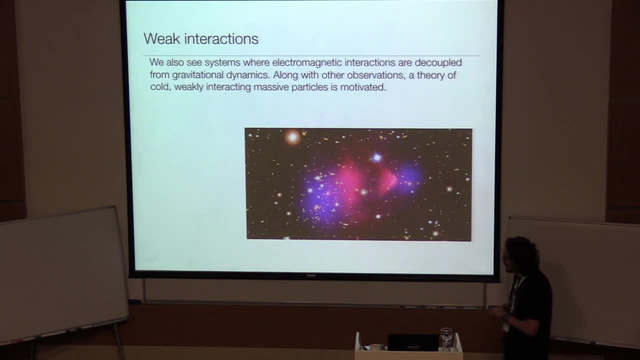 which I hopefully will eventually define. But you rely on gravitational lensing to say, OK, there's this amount of matter along that line of sight And just integrating that, you figure out that there is a lot of mass that is not impeded by this collusion. 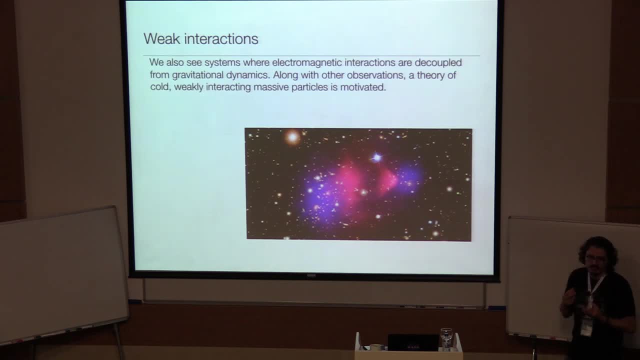 Now, what this means is the clusters essentially have two mass components, one of which is collusional, the other is collisionless, But at least has a really large limit, or small limit, tight limit, on its ability to collide. So that is yet another property that we expect from dark matter. 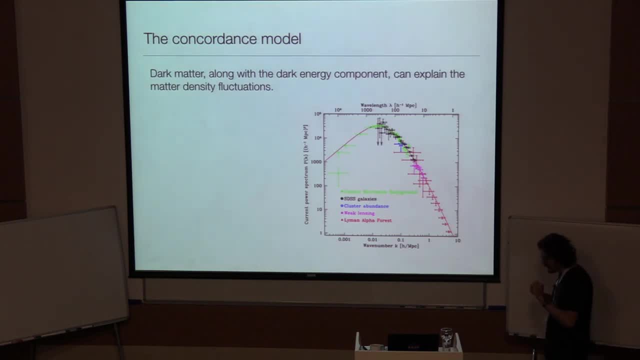 So bringing those ingredients. so the dark matter that I've already talked about. I haven't really mentioned the dark energy, But let me just spend a minute on it, just so the picture is complete. So in the last 20 years we've- I. 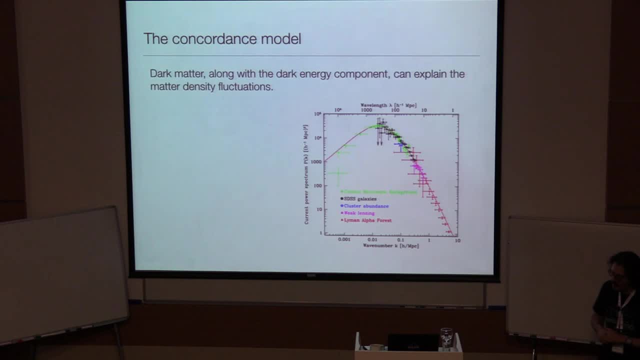 think you've already listened to many talks, or maybe even heard them in the news, But we know that the universe is expanding in an accelerated rate And that basically comes from Type Ia supernova data. So we just look at the luminosities of, or rather, 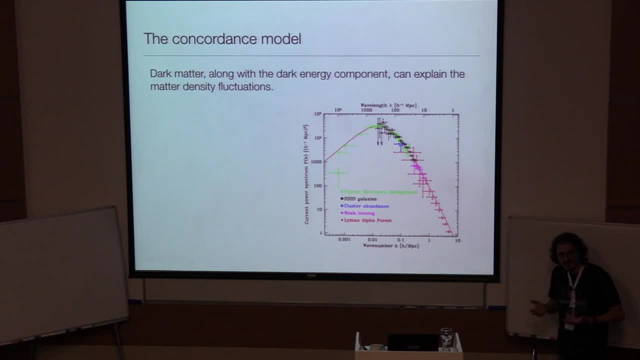 the brightnesses of the Type Ia supernova. And just because they're standard candles, that is, they have a standard luminosity, we can infer, we can infer the distance to them And by just laying out those distances you figure out as a function of redshift. 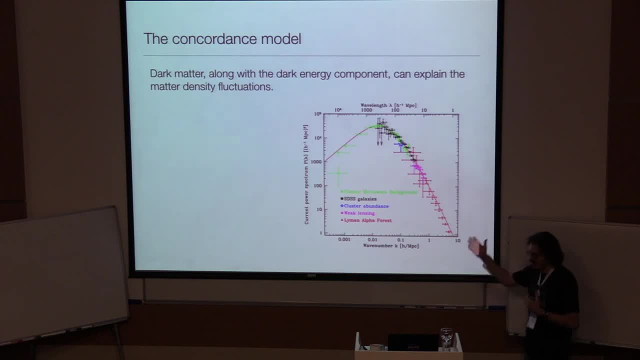 what's the acceleration rate of the universe And that tells you basically the acceleration history of the universe. And in order to be in agreement with your observations, we need to postulate an additional component which is homogeneous across the universe. So it's not like dark matter which is clumpy. 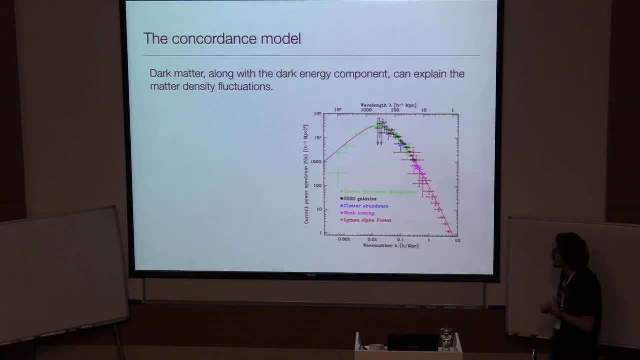 Dark energy must be. It must be almost like, homogeneous, like the vacuum energy with a negative pressure, So it actually accelerates the universe as opposed to collapsing it. So there has to be an additional component which, by the way, 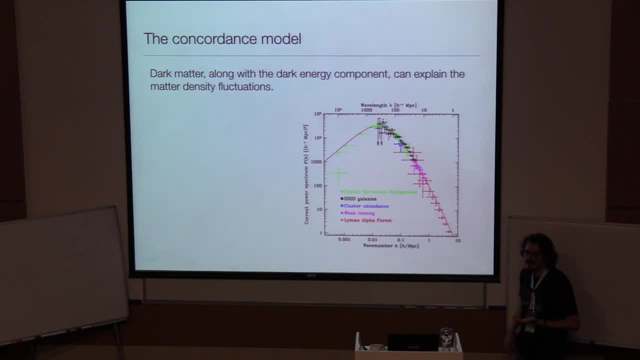 in energy density is even larger than the dark matter. It's about 68% of the universe, Anyway. so, bringing those two together and also the matter that we know and love, the baryonic matter, And in addition there is well, I also 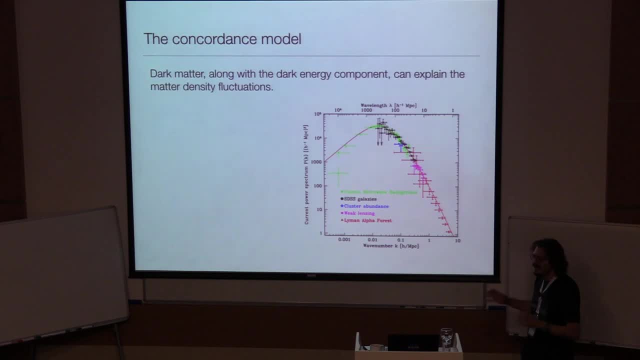 have to mention. there's the neutrinos and the photons. There's the neutrinos, There's the radiation. Bringing all of these together, we now have a cosmic chart of the energy budget And that's called the lambda CDM model. Lambda stands for the dark energy. 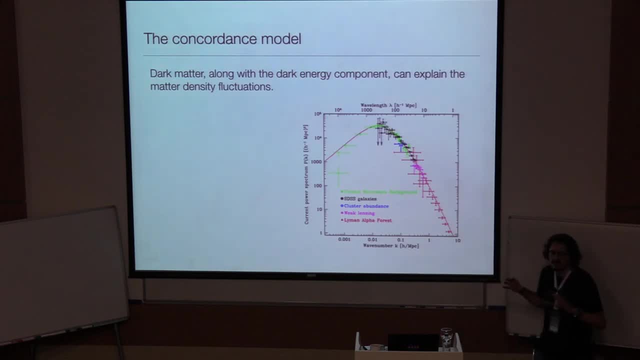 CDM stands for cold, dark matter. So that's the standard model of cosmology today, And this plot by Max Tegmark basically shows the various data points that show agreement with this lambda CDM model. On the left-hand side you have 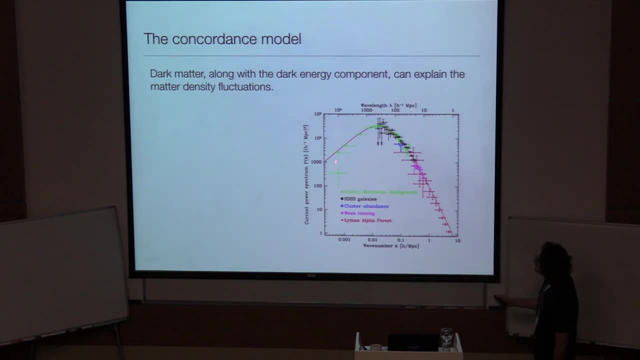 On the right-hand side you have the largest scales, like the CMB scale, so these green data points- And on the right-hand side you have the smallest scales. These basically come from the Lyman alpha forest, And then you have weak-lensing measurements. 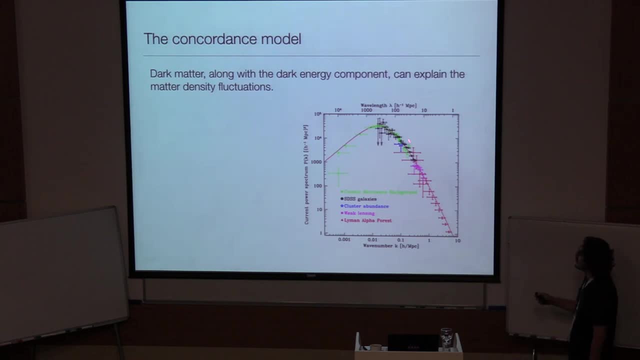 and basically counting clusters in the universe And also the picture I was just showing, the spectroscopic picture. these surveys essentially count galaxies in the universe And you have a collection of data points which agree with the prediction of the lambda CDM. 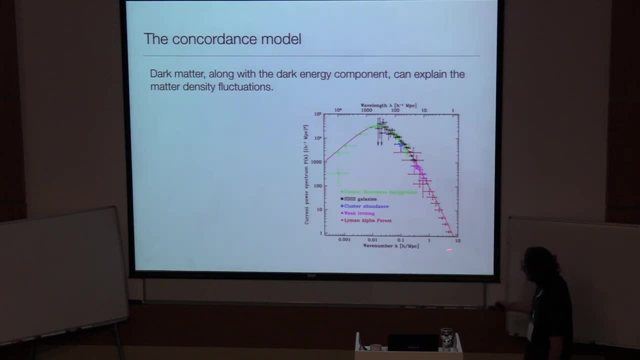 And then you have a collection of data points which agree with the prediction of the lambda CDM, And I haven't even defined axes, sorry, This is wave number, so inverse distance, And this, basically, is the power spectrum associated with it. 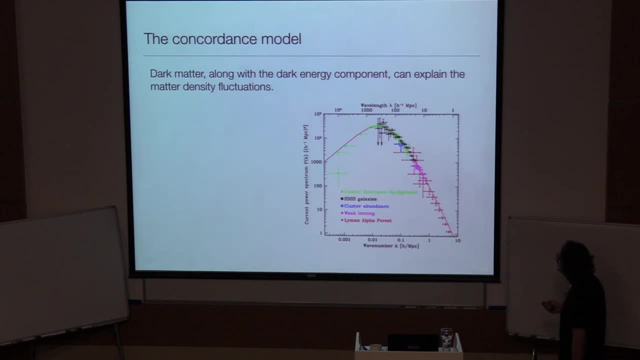 Again, just power as a function of wave number. So we now have a great agreement between observation and lambda CDM. that makes us very happy. But there are still problems with lambda CDM, which I will come to in the fourth lecture. at very, very small scales. 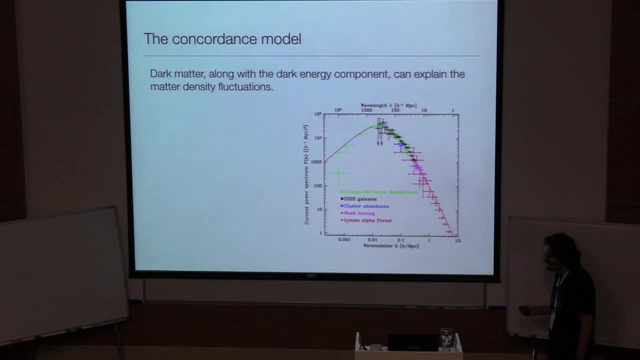 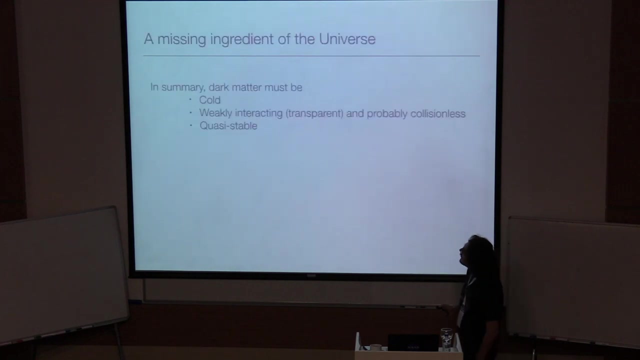 But it actually doesn't make sense to point to the right In this plot, because this plot assumes linear growth like this is wave number. However, at some point when structure grows in the universe, it becomes nonlinear after certain points. So we will come to that as well. 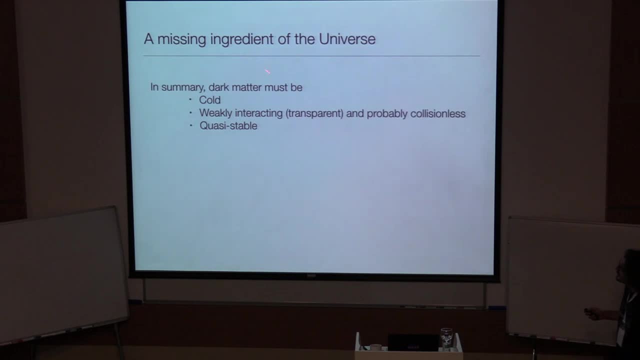 However, before I talk about structure formation, just one thing, just summing up the story now: Dark matter must be cold, So I haven't really defined cold. Cold means non-relevance, Cold means non-relevance. Cold means non-relevance. 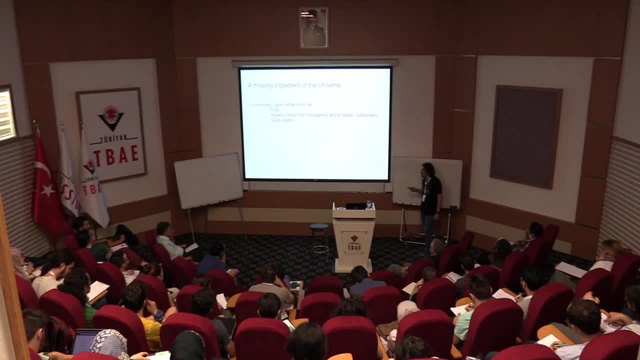 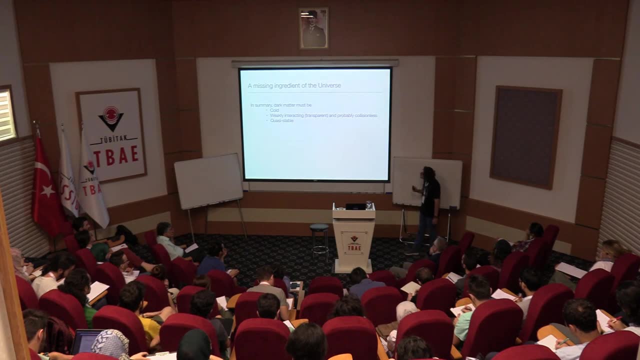 Cold means non-relativistic, But we want it to be cold not at an arbitrary time, but at by, or I should say by, not at, but by the CMB- Sorry, CMB's recombination- So by the production of the CMB, or rather, putting it in a different way, by the epoch of recombination. We want it to be non-relativistic, just because if it was relativistic it would just be like radiation And it would dilute. It would dilute away the density contrast. 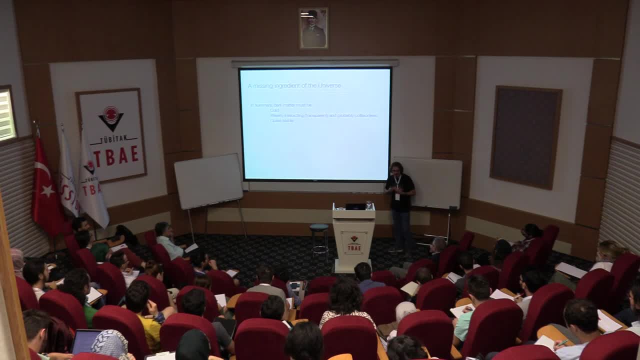 So if you want to grow structure, you want a non-relativistic component. That's the key point here. Second, you want it to be weakly interacting. I think I have motivated this point enough by showing the bullet cluster, And by that I really mean it's transparent, not dark, not. 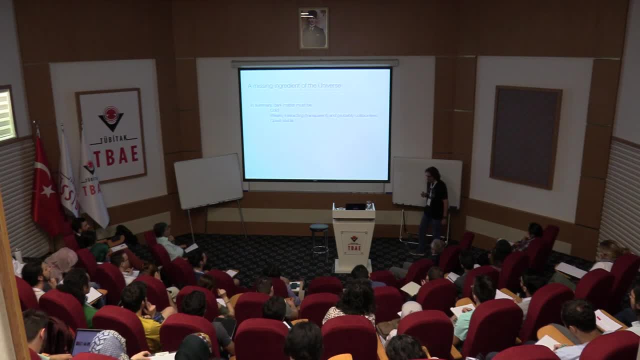 black. I think a transparent matter would be a better name for dark matter. However, dark just means or is a dark is an adjective that conveys our ignorance about it, So I think in that sense it's fine. So dark energy is dark in the same sense. 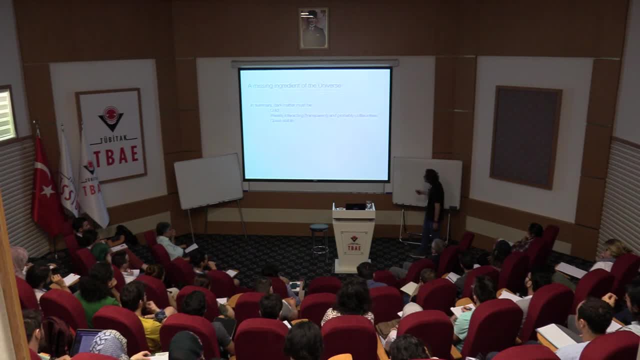 that we don't understand it And it's probably collisionless. I just said probably, just because there are also models of dark matter in which you have some level of collision in the model, but not very much Because there are limits on it. 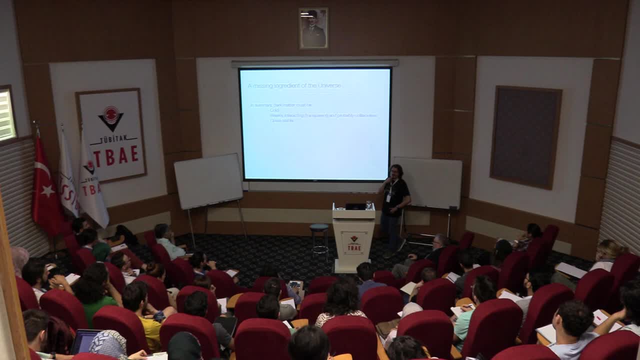 And it must be quasi-stable. By that I mean dark matter shouldn't decay, Because if dark matter did decay then it would not address your cosmological problem, Because it could solve your problems in the early universe. It could solve your problems during the dark ages. 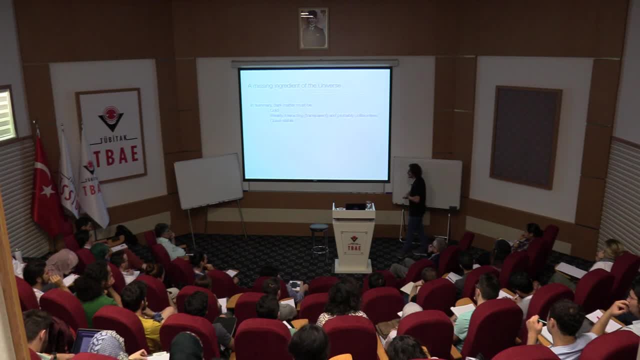 But it wouldn't solve your problem today, Because by the late universe you would have structure just diluting away, And you don't want that to happen. There are many dark matter models in which the dark matter particle is quasi-stable, That is, it's not like proton, which 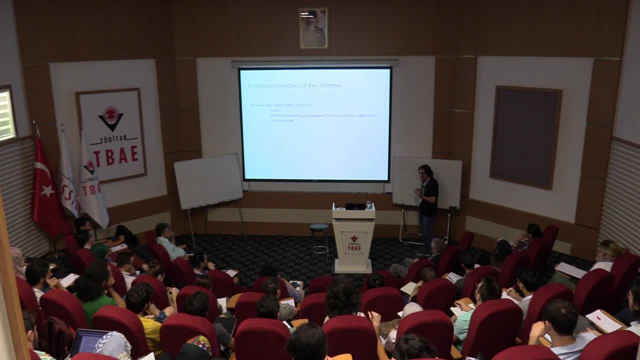 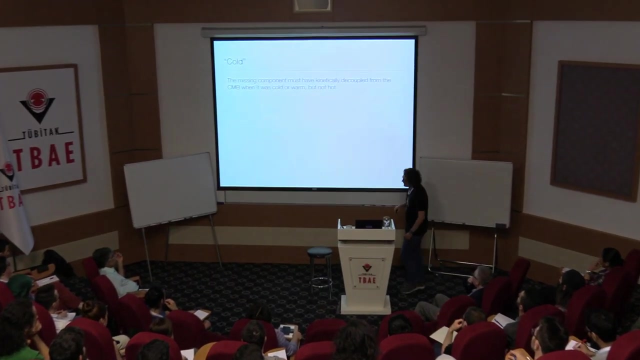 has a lifetime of like 10 to 34 years, But it basically can live up to Hubble time And maybe in a few billion years the dark matter will start decaying. Maybe We don't know. Oh OK, I have some slides. 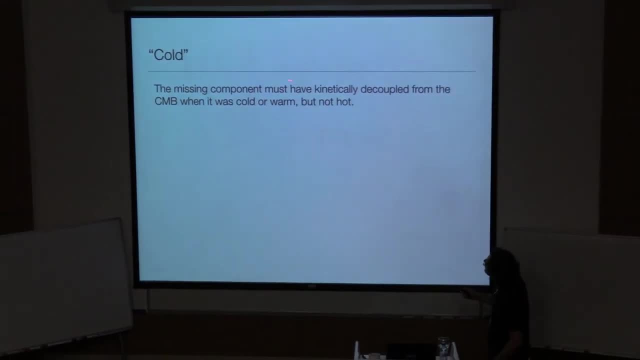 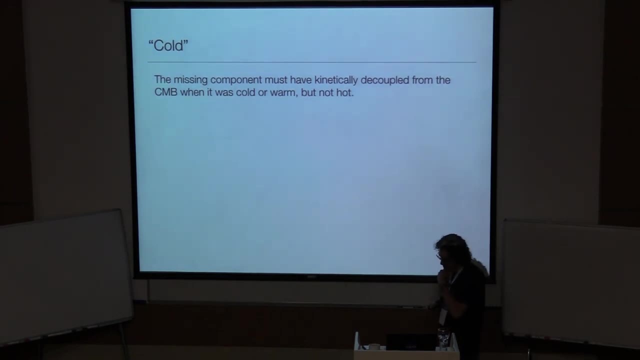 But I think I've already mentioned Yes, maybe I just didn't say kinetically decoupled, So I've, When I say OK, Recombination, I think I should be more precise here, So I said epoch of recombination. 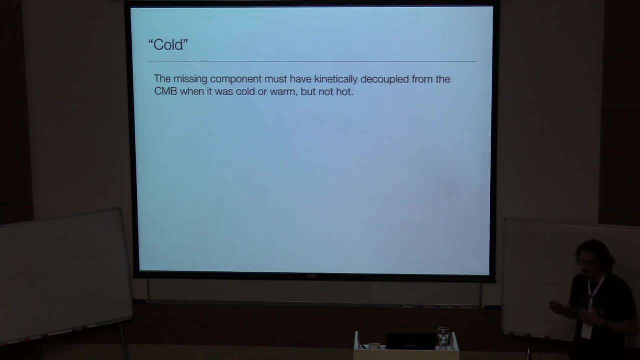 But we really don't know when dark matter actually decoupled from the rest of the cosmic plasma. So, technically speaking, we really want it to be cold. that is non-relativistic. when it's kinetically decoupled from the rest. 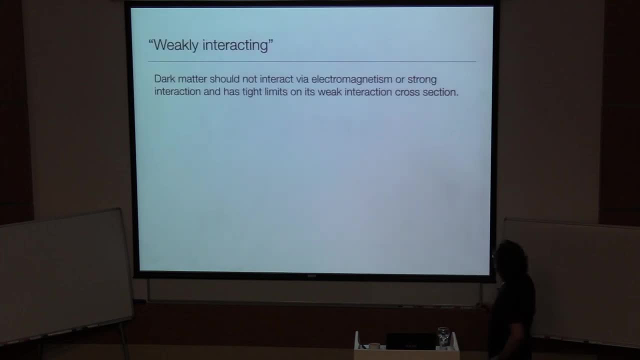 of the cosmic plasma. That's a better way to put it, And we certainly don't want to be hot. That's non-relativistic. It can be warm. By warm I mean it can basically have a free streaming length that is comparable if you basically project that distance. 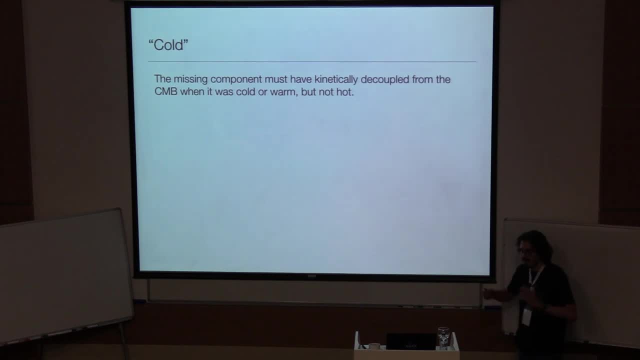 to today's standards You can have a free streaming that is of order, the dwarf galaxy size. But you don't want that distance, the free streaming distance, to be larger than that. Then you would be erasing structure that you actually observe today in the universe. 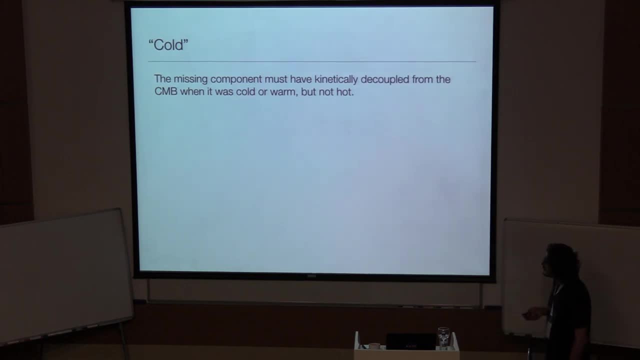 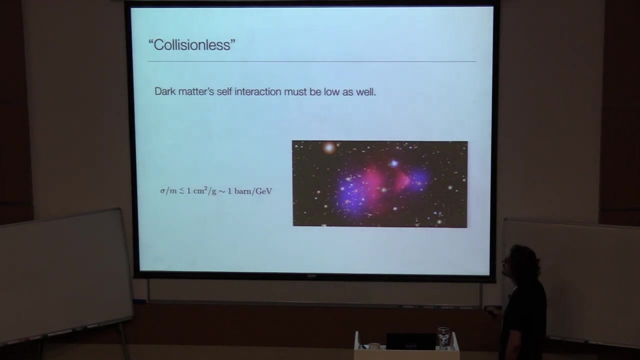 That shouldn't happen. So this warm dark matter is usually modeled by sterile neutrinos. I might say something about that later on, And I also mentioned this weakly interacting. I'll pass that. So the self-interaction must be low for the same reason. 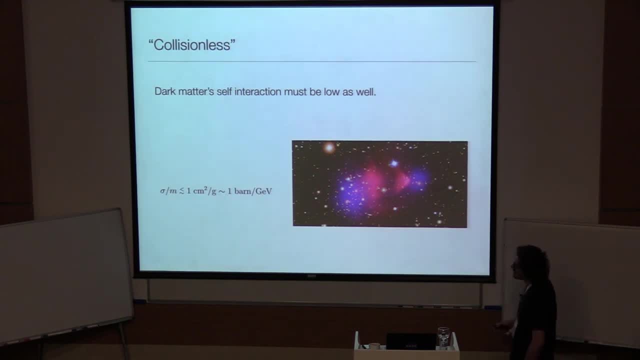 Just to quote a number that's a very useful number to remember. It's about a barn per GeV, the cross-section that you allow. Anything lower than that is fine, But anything larger than that you start not producing the bullet cluster. 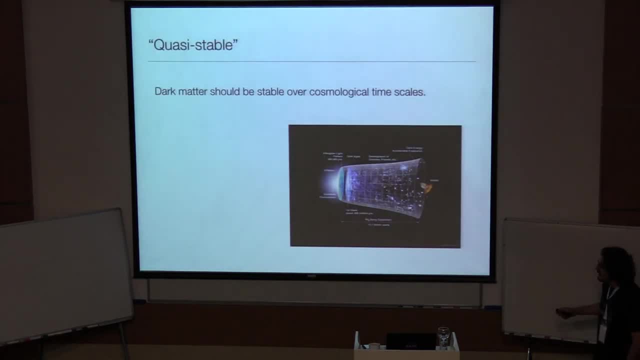 That's no good And it must be quasi-stable for reasons I mentioned. So we sit here at the moment. That's the epoch of recombination. That's basically the inflation, And dark matter can essentially decay any time in between, But it shouldn't completely decay. Completely decay, at least by now, Otherwise it wouldn't solve the dark matter problem. So one thing I should probably mention before going into the particle nature: Does it imply that dark matter does not interact gravitationally among itself? No, dark matter does interact gravitationally. 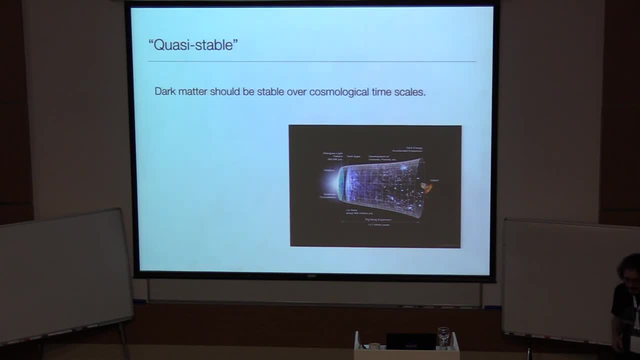 It interacts gravitationally with the other matter, the ionic matter? Yes, Does it interact internally self-gravitational. So Self-interaction can happen, but only So there is a self-interacting dark matter model. But there is actually an upper limit to its self-interaction. 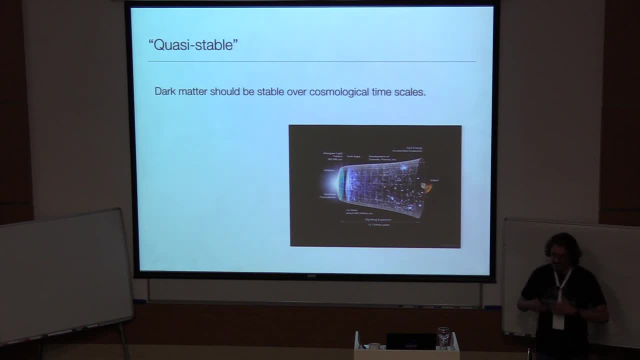 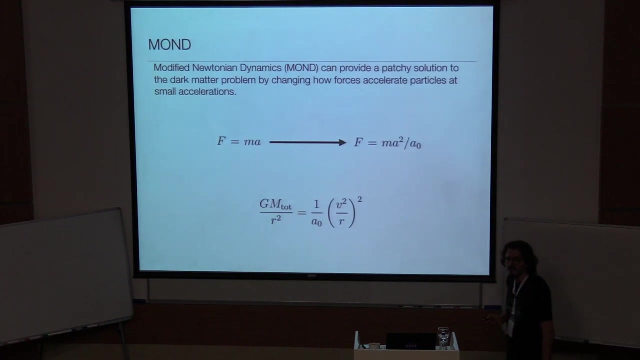 However, by self-interaction we don't mean gravitational. Gravitational interaction is common, So gravitational interaction is true for baryonic matter as well as dark matter in the same sense. Yes, Sorry, two questions, Let's go one by one. 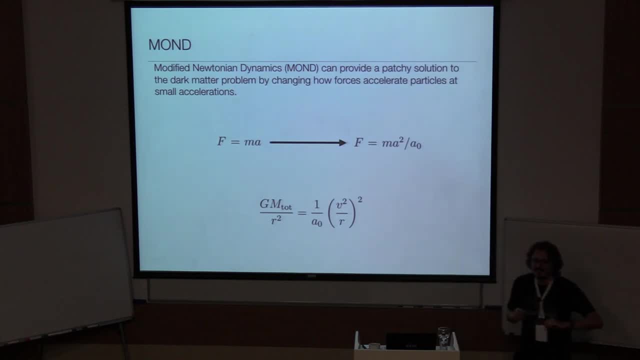 Sorry, who was asking the question? I missed You. OK, What do we know about dark matter before the recombination, Before, Yes, Do we know something about dark matter Well prior to recombination? the only observational evidence we have is the Big Bang nucleosynthesis. 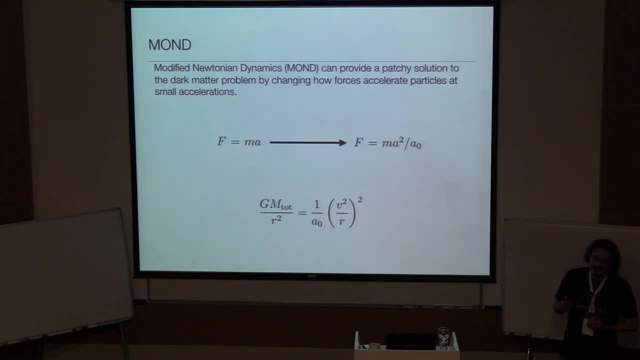 And that only tells us. It tells us about the baryonic abundance. So we learn pretty much all we know about dark matter from either current galaxies by just studying how fluffy they are, et cetera, the rotation curves, et cetera. 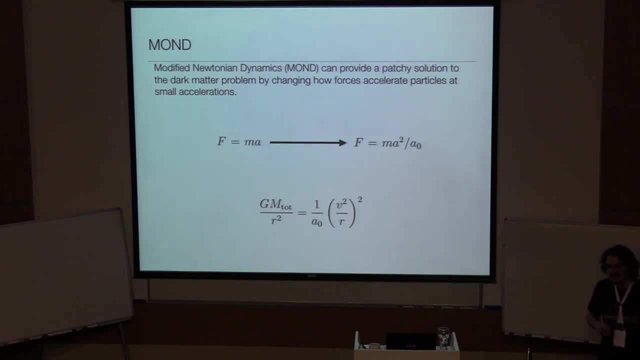 the abundance of galaxies, But these are all late time effects, And also the CMB, But I mean only observational effects. There are many models. I'm not referring to the models, I'm referring to the dark matter themselves. We know a lot. 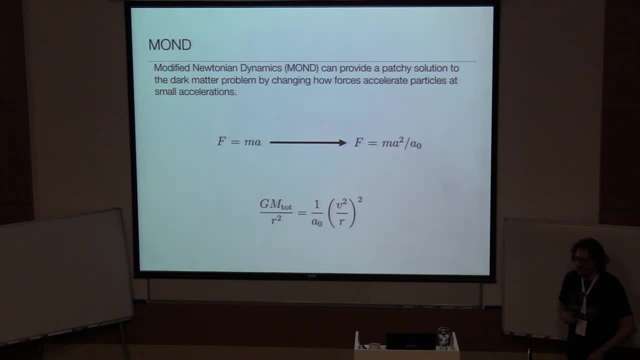 So what you meant by knowing is the number of models we have. We have zillions of models about what dark matter could be doing. OK, Yes. What about peculiarities of safe, interactive dark matter models? What are what Peculiarities? 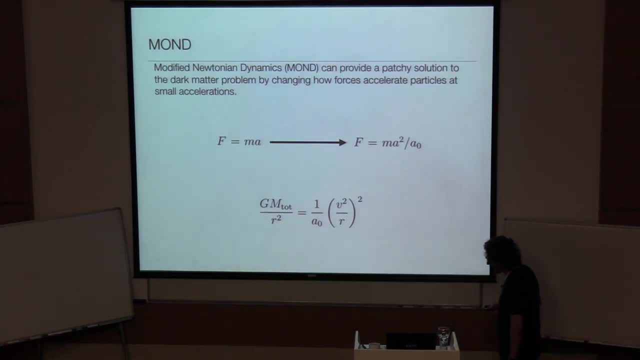 Well, if dark matter self-interacts, first of all, it would The most obvious result. It would be to erase structure at smaller scales. In lambda, CDM, in cold dark matter scenarios, matter starts clumping at the very, very small scales. 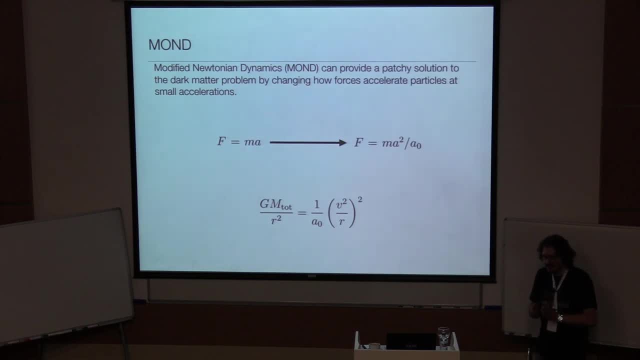 Obviously, there's always a finite free streaming for any type of component, including dark matter, But that free streaming length is extremely small. So in lambda CDM you may have clumps as small- It's as small as the Earth itself. 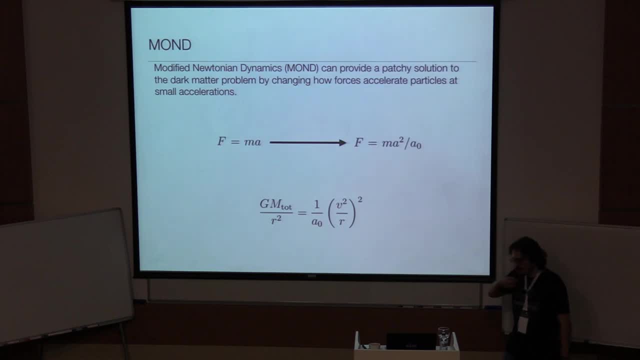 Like pretty small, I mean. However, when you introduce self-interaction, that starts smoothing out those structures. So basically, you end up with a universe that very much looks like the warm dark matter model, with certain differences, Because when you have interactions, 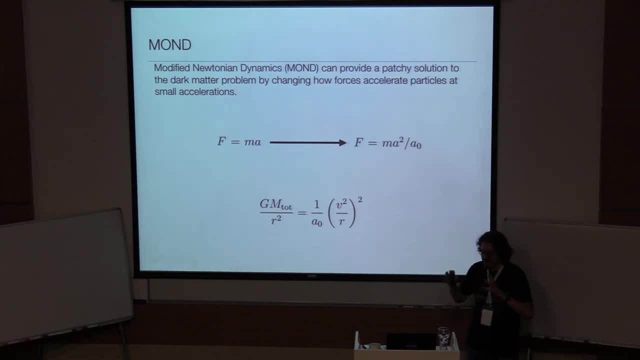 it also changes the sphericity, Like there might be triaxiality et cetera, But those are always secondary effects. The most obvious one would be erasing the structure. OK, So erasing the structure, That has basically implications also. 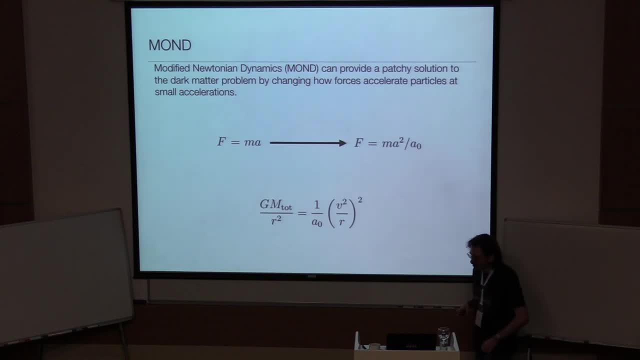 for indirect detection of dark matter, Because it changes the number of clumps that you expect to exist And that changes the amplitude of the annihilation signal that you expect. So it's like a pipeline that feeds into the indirect detection as well. 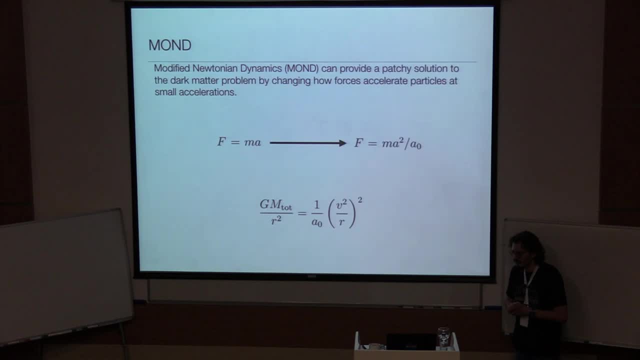 So do we have, Do we have, rigid evidence that dark matter has structure? Well, the evidence we have is CMB+. It has to have at least the structure that the baryonic matter has, Otherwise, I mean, both are gravitationally interacting. 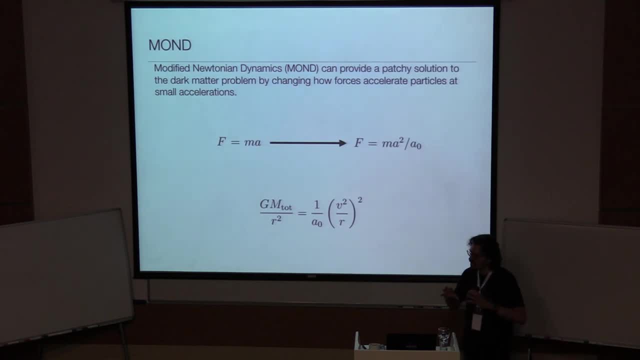 So at least that must be the case, But I think you are referring to structure that is smaller, for example, than the dwarf structure, So it's not the size of the galaxies et cetera That we don't actually have. That is an extrapolation of the model And we don't have evidence. The smallest structures that we see are these dwarf galaxies, the smallest dwarf galaxies in the local group that we have observed. They have masses of order 10 to 6 solar masses. a million solar 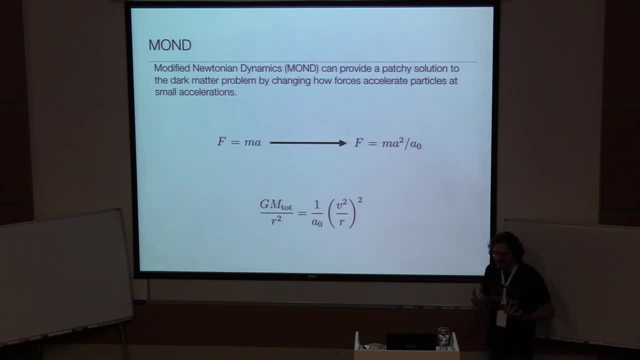 masses, But that's it. Anything lower than that. we just don't have evidence for Dark matter is, say, completely decoupled. It doesn't interact with the standard model of whatever we know about a standard model. Do we have any hope to probe what it is? 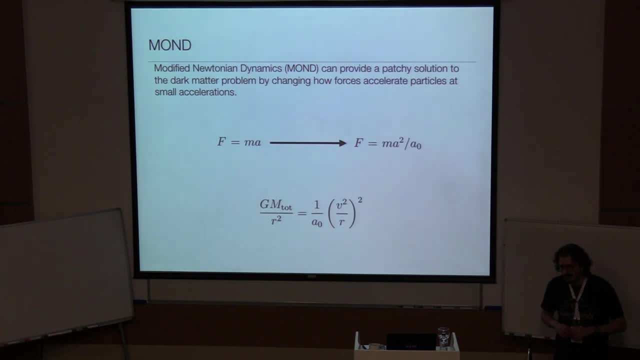 other than only gravitationally? Probably not. Yeah, Like gravity knows. Yeah, Yes, please Sorry. Could I add something to that answer? Yes, please, Yeah. So there's a class of models where you have supersymmetry. 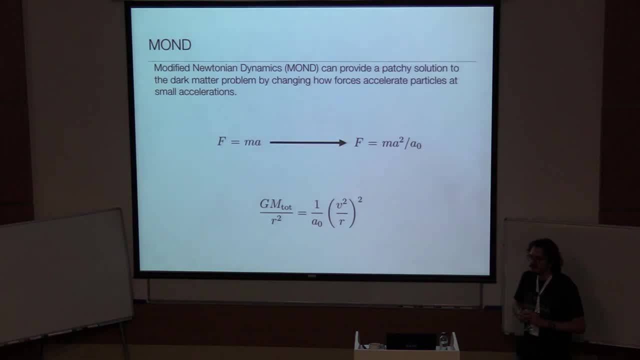 And the gravitation is the lightest supersymmetric particle. So in those models the gravitation is the dark matter, It is a so-called super wind, It only has gravitational interactions, And you can never discover, However, a property of those models. 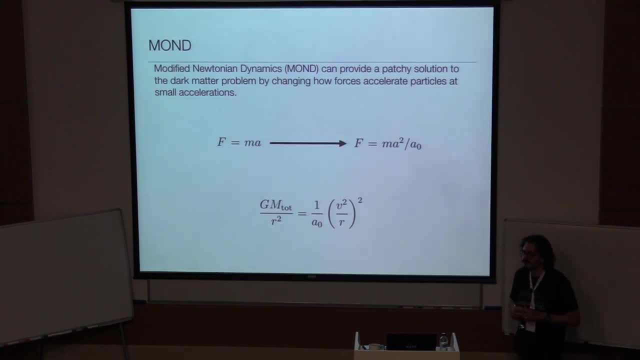 is that all of their supersymmetric particles have decayed in the gravity, sometimes rapidly, And so by discovering supersymmetric particles and analyzing their decays and seeing this particular regularity, you can actually directly discover the gravity. So you have to really look at the whole model. 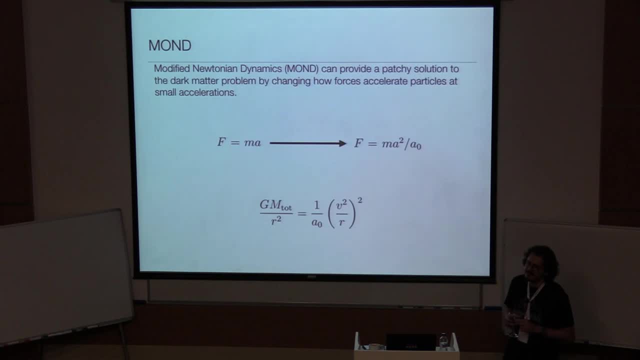 and see what its implications are before you say it can. Yeah, good point. I guess everyone has a different definition. Some people like to see actually the particle itself just decay Or something. But I think that's a great point. Sometimes the models have some degeneracy. 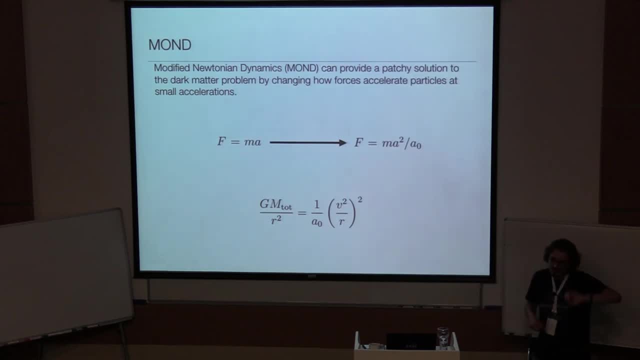 So you have to actually constrain it from some other direction and just indirectly infer the existence of a particle. I think that we discovered the tau neutrino as soon as we discovered the tau weapon. Yeah, Because there's something missing And it's highly constrained. 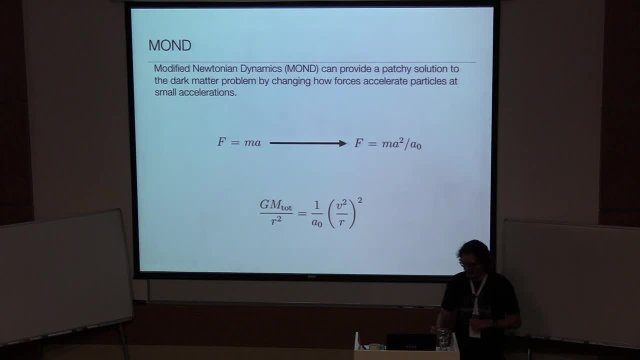 So what else can we do? Yeah, Now other people claim that the tau neutrino was discovered 20 years later, And so I think this is the right answer. Right, Yeah, Yeah, Was there a difference? Yes, As being the lightest particle, as you mentioned. 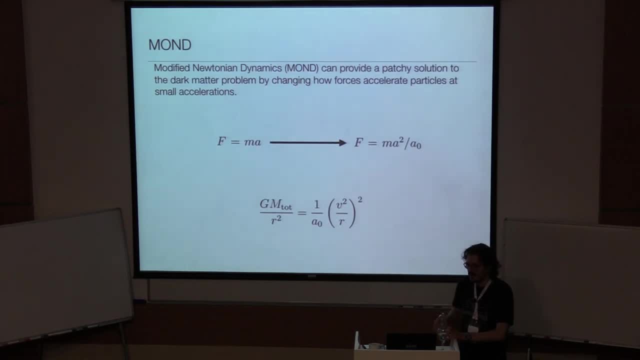 isn't being non-relativistic, isn't it a contradiction? OK, But so dark matter is probably so dark matter. for example, talking about the weakly interacting massive particles, It has to be non-relativistic And it's actually very massive. 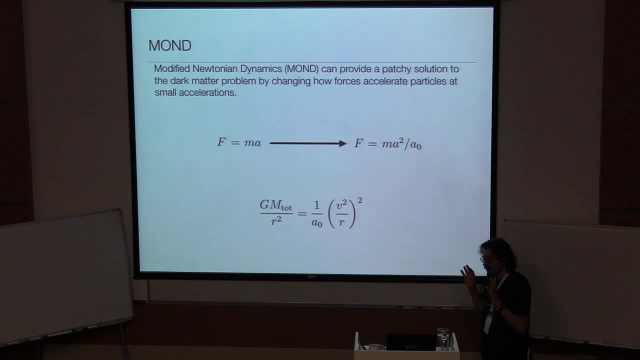 It's like 100 GeV. So there are lighter light bosons that can make up dark matter, But they behave very differently Because they're non-thermal, They're bosonic. Their model is very different. They behave like waves. 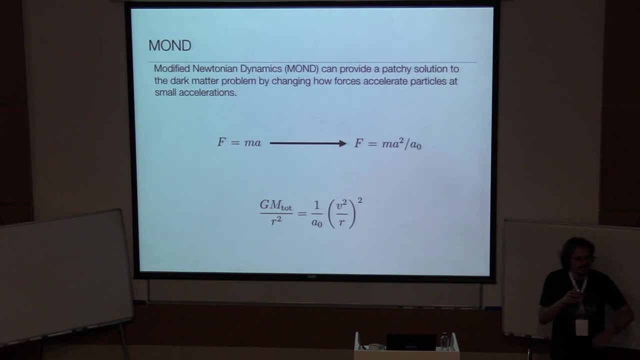 They're not like fermions. Yes, But I thought there's a scale problem of lambda c that has hand core problems And the light dark matter can solve this problem. to smooth out, to produce a core, Yes, And what do you think about this problem? 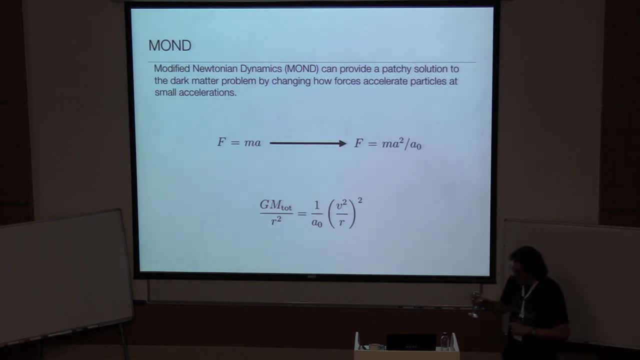 Yeah, Yes, So actually this will be the main topic of my fourth lecture, But certainly let's just discuss that real quick. So there are many solutions to this core cusp too big to fail and missing satellites, problems of lambda, cdm at small scales. 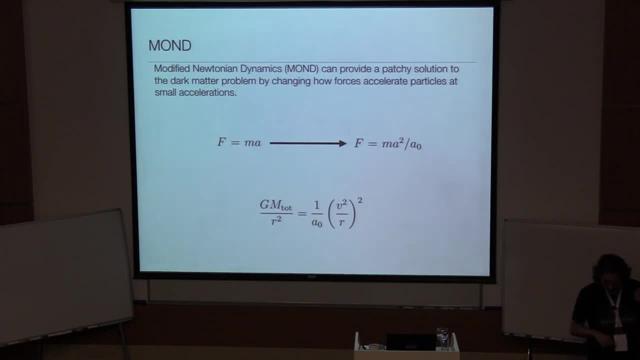 One solution is self-interacting dark matter. Another solution is warm dark matter, where you introduce some temperature to the dark matter at kinetic decoupling, And these are all fine. I mean certainly they can be a reality. Or there's wave-like dark matter, as you mentioned as well. 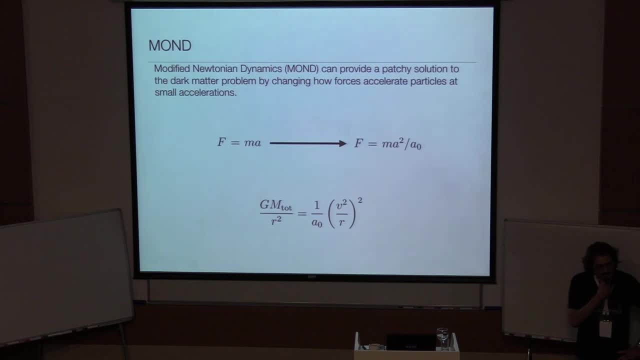 I think at the moment no one knows which one is better. We certainly haven't singled out one of them, That's certainly true. But I would even argue further that we don't even know which one is a better candidate, Because this is a really old problem. 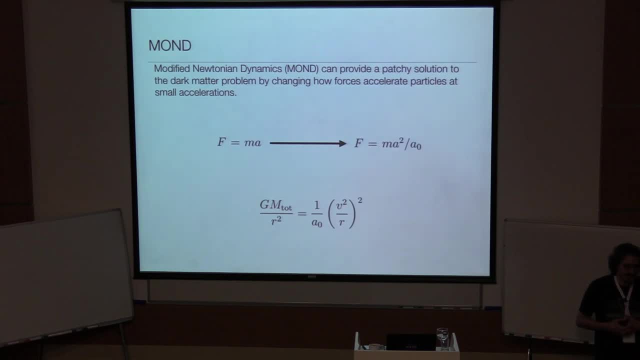 but a problem that lacks very much observational data. So for a long time people have written papers based on their prior beliefs rather than the method effect. So I think all these models are certainly possible And I really wouldn't claim one better than the other. 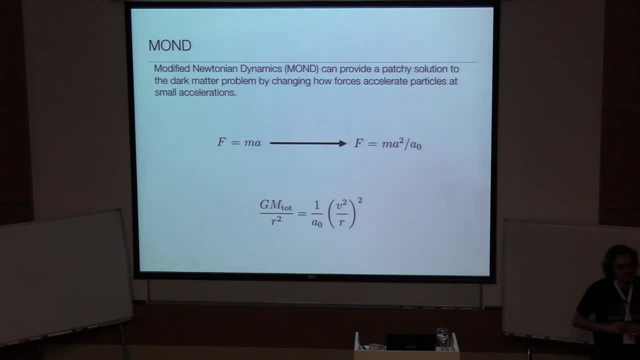 What about computer simulations? Is it possible to distinguish by using the simulations? Well, computer simulation is for forward modeling the model. So for every given model you can start a hydrodynamical simulation that forward models your whatever initial condition is. 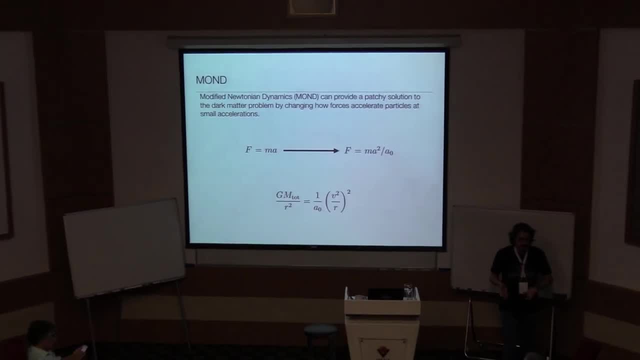 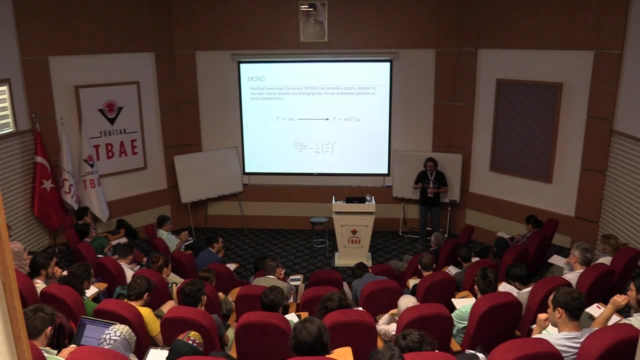 And pretty much all these models that I enumerated can solve the problem in different versions, So they're kind of degenerate. Unless we get a particle, basically a signal, from the particle nature of them, it may be even impossible to distinguish, And so wave-like dark matter behaves slightly different. 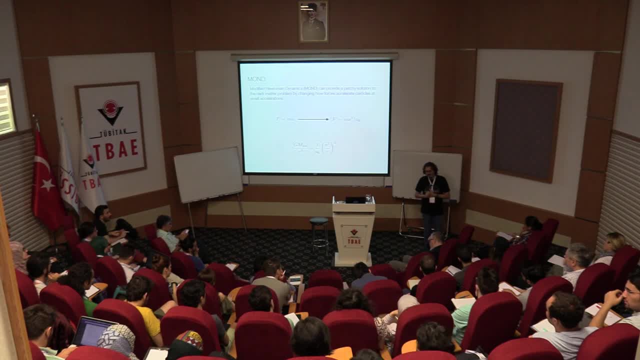 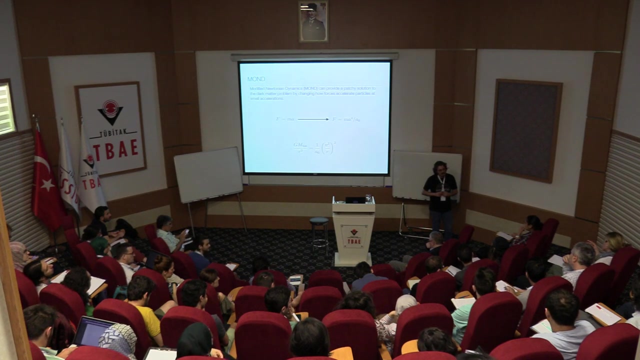 So I would say wave-like dark matter is slightly different than the others. So the self-interacting one and the warm dark matter one, I think, look very much similar. It's really hard to distinguish those two. No, actually it doesn't have to interact. 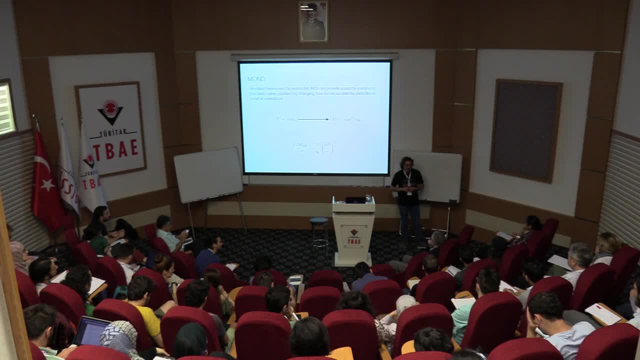 So warm dark matter, a good candidate for warm dark matter- is sterile neutrino. A sterile neutrino is a neutrino that doesn't interact weakly. So active neutrinos that we know and love basically interact gravitationally and also weakly. 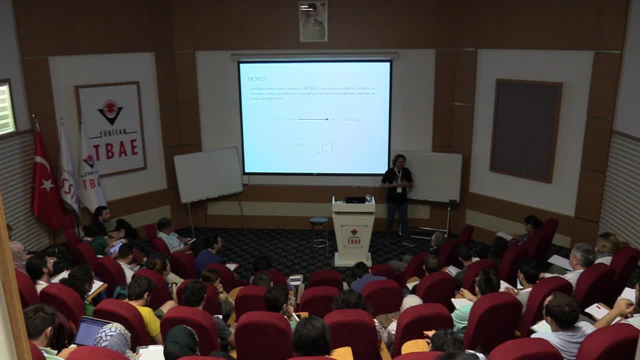 Sterile neutrinos don't interact weakly, They only interact gravitationally, And they're much more massive. Well, we think if they exist, they must be massive. They're like keV, kiloelectron-volt kind of mass.